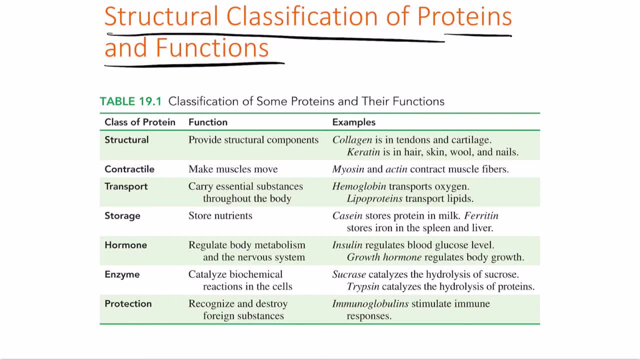 classify them based on their functional properties. First class of proteins is structural proteins, So first class is the structural proteins. These are structured. these provide the structural components. Main two of them are collagen, collagen and carotene. Collagen is the one that is present in tenders and cartilage. 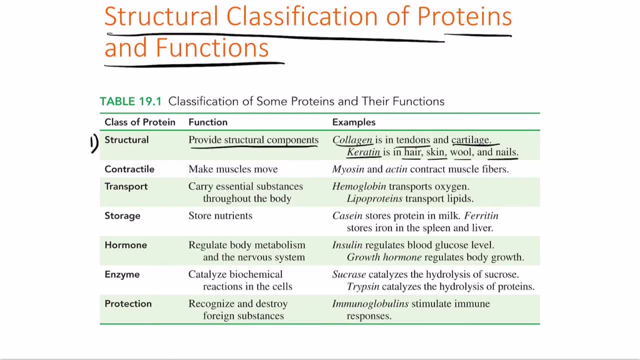 Carotene is the one that is in hair, skin, wool and nails. Next you have the second one: contractile muscles, Contractile proteins which are made, which make the muscles move. So there are two of them. one is myosin and actin. So they try to. 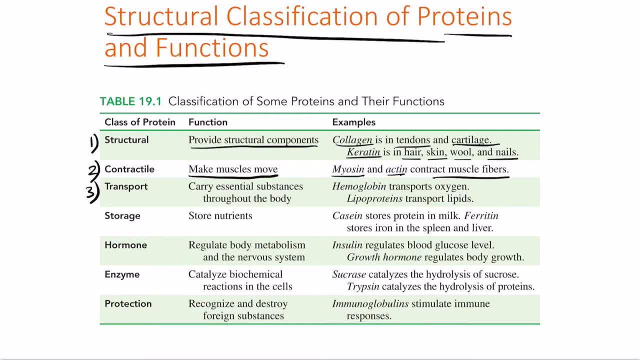 contract the muscle fibers. Next, you have number three: transport proteins. These are the ones that carry essential substances throughout the body. There are two of them, mainly hemoglobin and lipoproteins. Hemoglobin transports oxygen. lipoproteins transports lipids from lipids through non-polar, polar substances. Number four: 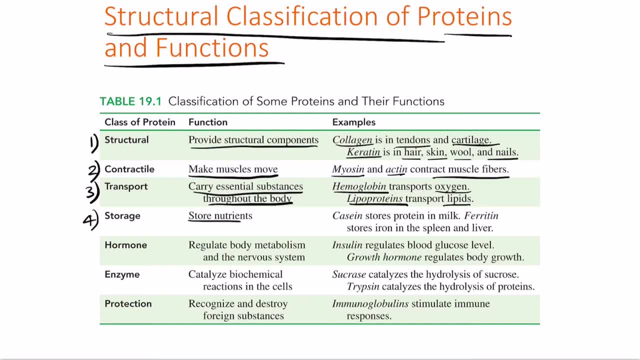 you have storage proteins. These are the ones that store nutrients. One of them is casein, which is the protein in milk stores protein in milk, and ferritin, which stores iron in the spleen and liver. Next, you have number five: hormone proteins. These 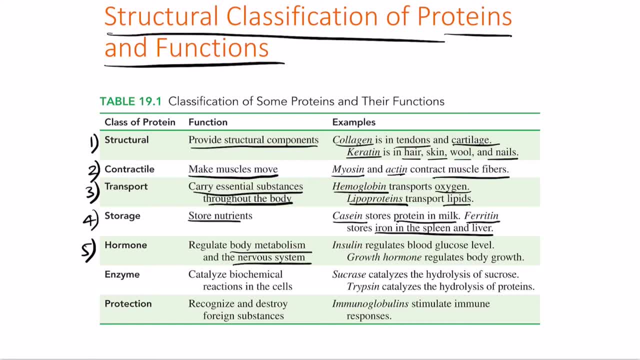 are the ones that regulate the body metabolism and the nervous system. For example, one of them is insulin, which regulates the blood glucose level, and the other one is the growth hormone, which regulates the body growth. Next six, you have enzyme, enzymatic proteins, which are the catalysts of biochemical 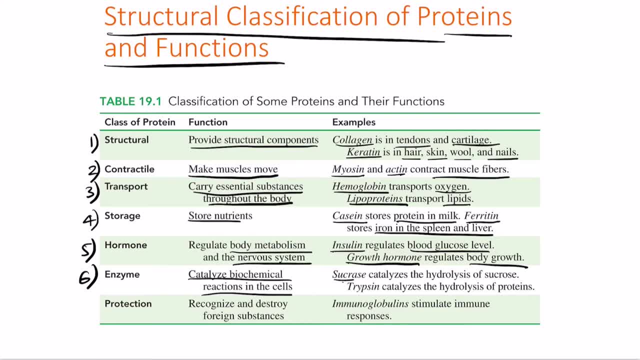 reactions in the cells. So two of the two examples would be: sucrase is the enzyme that hydrolyzes sucrose. Trypsin is the enzyme that catalyzes the hydrolysis of proteins. Next, you have seven protection proteins. These are the 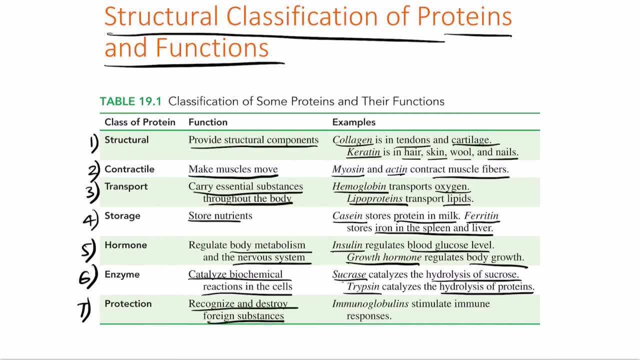 ones that recognize and destroy foreign substances. so best example of these are immunoglobulins. these stimulate the immune responses in your own body. So proteins have varying purposes and they generally do very, very different tasks from one another. so proteins are made from the building blocks. so the building blocks of proteins that are made from an amino acid. so the protein was made from the building blocks of proteins that act as marker. so the enough of proteins to remove the polymer r grupo, that's paper and body, is the main component which his 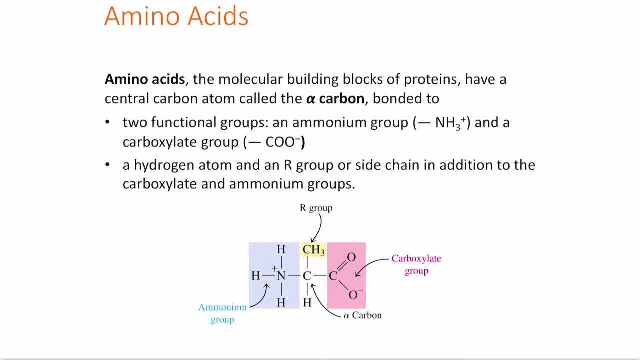 Ф все. the building blocks of proteins are amino acids. so amino acids are the molecular building blocks of proteins and they have a central carbon atom- we call it the alpha carbon- and bonded to two functional groups- remember the term: amino and acid. so the name comes from the fact that it actually 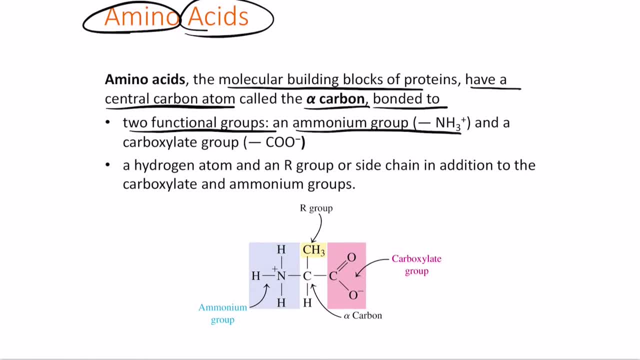 is connected to two different functional groups. it contains an ammonium ion, which is nh3 plus, and a carboxylate group, coo minus, and a hydrogen atom and an r group on the side chain, in addition to the carboxylate and the ammonium groups. so this is the alpha carbon. you have the carboxylate. 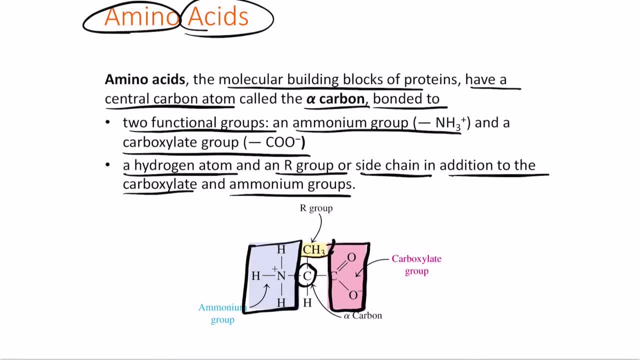 group you have the amine group and on the top you have an r group. r group can be any one of these structures. r group are different structures based on the different protein, but on the other side there is always a hydrogen. so this is the one that varies from one type of one type of. 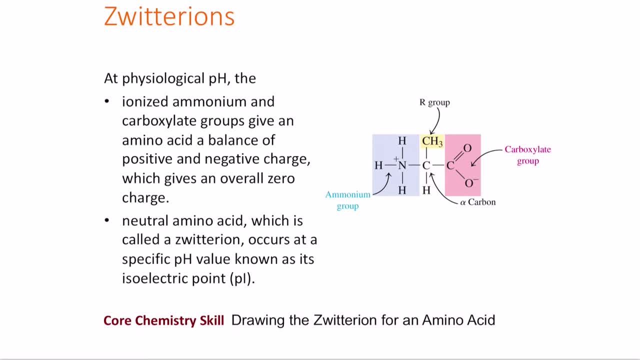 amino acid to the other type of amino acid. so at physiological ph, which is in the ph level in your body, the ionized ammonium and carboxylate groups give at the amino acid a balance of positive and negative charges which, when you consider it as an overall zero charge, because one is plus and 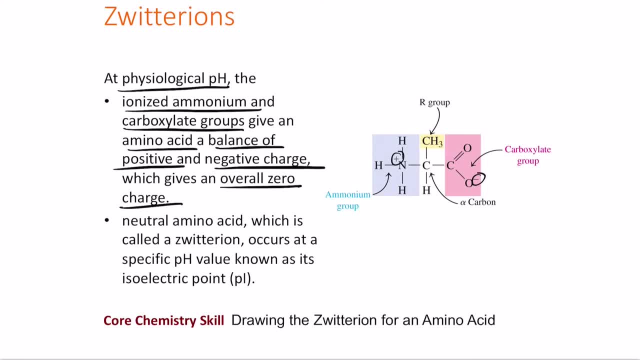 the other is minus, so it results in an overall zero charge. so this is called as a neutral amino acid, which is generally called as a zwitterion. so zwitterion is the structure that results in the formation of a carboxylate group. so this is a neutral amino acid, which is generally called as a. 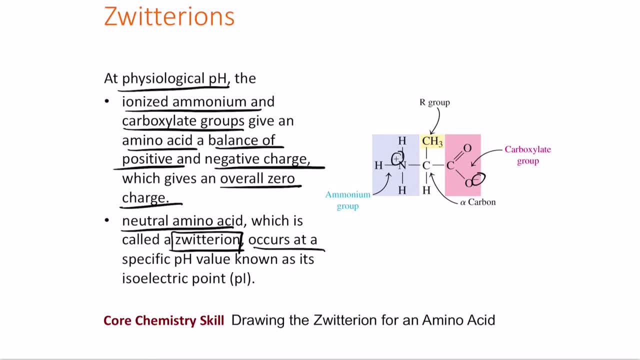 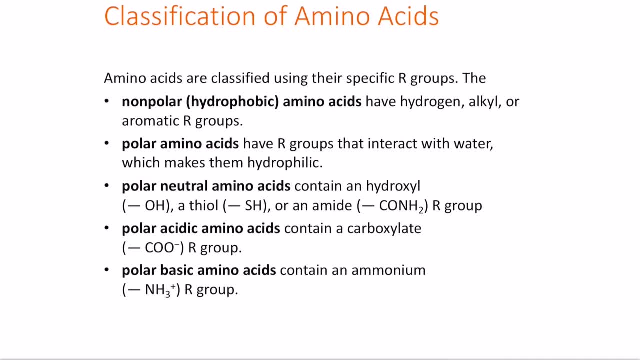 zwitterion. so zwitterion is the structure that results in the formation of a carboxylate group of a neutral amino acid, and it generally occurs at specific ph values. we call it the isoelectronic isoelectric point, or pi. so we'll talk more about it as we go along in the lecture. now, how do you? 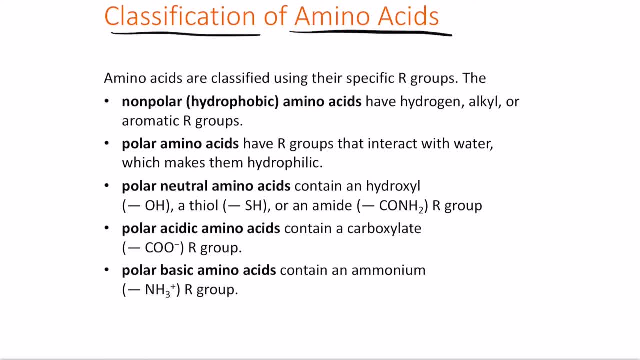 classify amino acids. so there are 20 different amino acids. we can classify amino acids using their r groups that are attached to the carb alpha carbon, so they can be non-polar amino acids, polar amino acids, polar and neutral amino acids, polar acidic amino acids and polar basic amino acids. so let's start with non-polar amino acids. 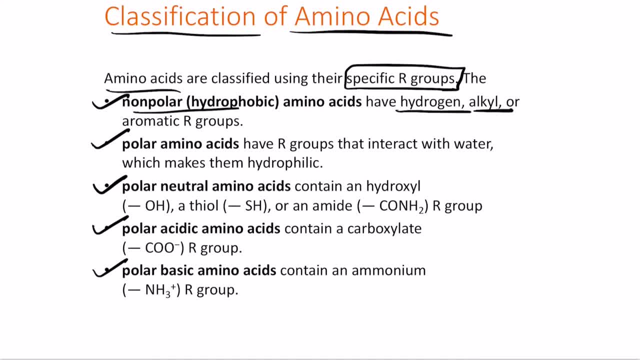 these are the structures that have either hydrogen alkyl groups or an aromatic r group attached to the alpha carbon. in place of the r group, here you have polar amino acids, which have r groups that interact with water and which make them hydrophilic. remember that non-polar means that these are 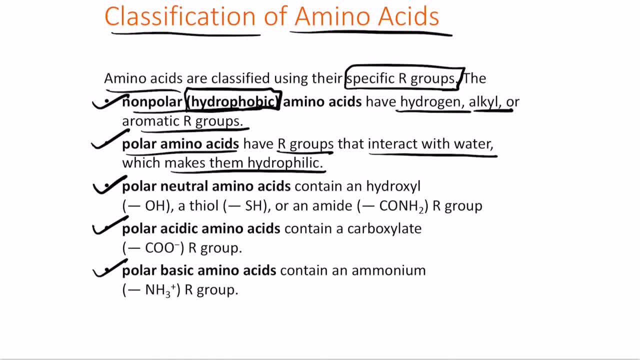 hydrophobic amino acids. hydrophilic are the ones that are polar amino acids. now let's start with polar neutral amino acids. these are the ones where the hydroxyl groups is neutral. example of them is hydroxyl group a, thiol, an amide as an r group. next you have polar acidic amino acids, which contains 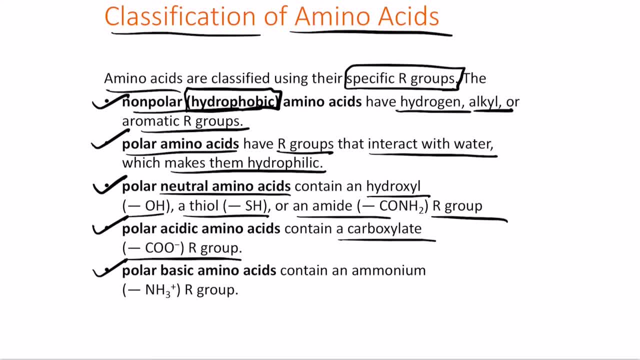 basically a carboxylate ion, another carboxylate ion attached to already carboxylated amino acid. you have a basic structure which contains an ammonium r group that is attached to the structure. so, in summary, there are 20 different ones, or 20 different one of them. 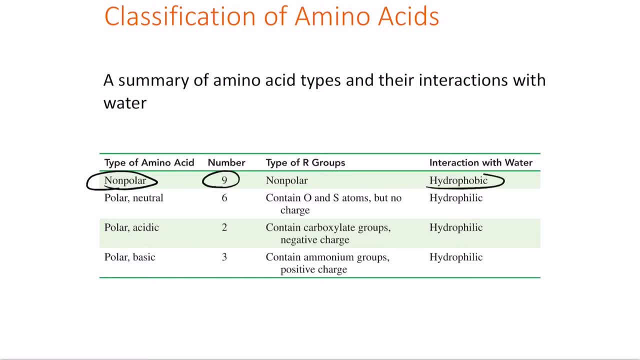 the non-polar ones. there are nine of them, and these are generally hydrophobic hydrophobic. the rest 11 are hydrophilic substances, and out of them, there are six polar substances that are neutral, two of them that are polar and acidic, three of them that are polar, and 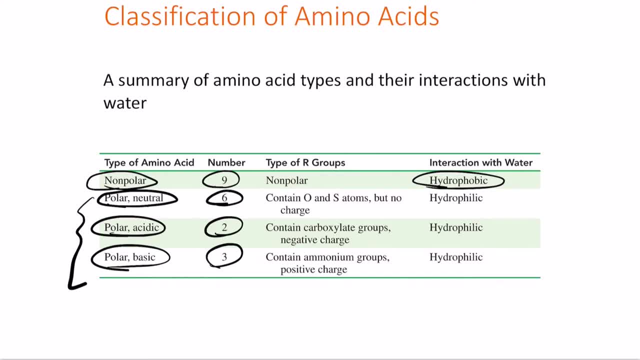 basic. so which ones are neutral? the ones that contain oxygen and sulfur atoms but without any charge. polar acidic substances are the ones that contain carboxylate groups and a negative charge, and ammonium groups and a positive charge, and non-polar groups generally contain non-polar r groups. 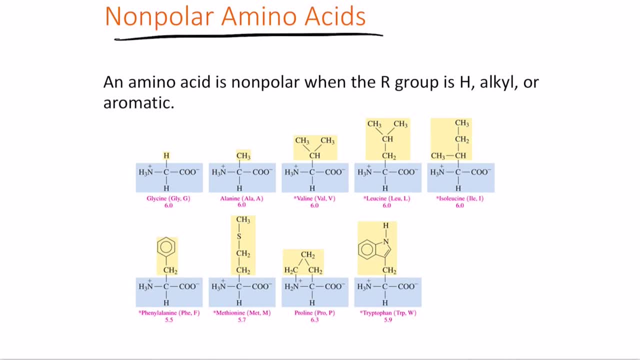 so let's start with the non-polar amino acids. these are the nine non-polar amino acids: glycine, alanine, valine, leucine, isoleucine, phenylalanine, methionine, proline and tryptophan. so these are the non-polar groups. notice that all of these, the r. 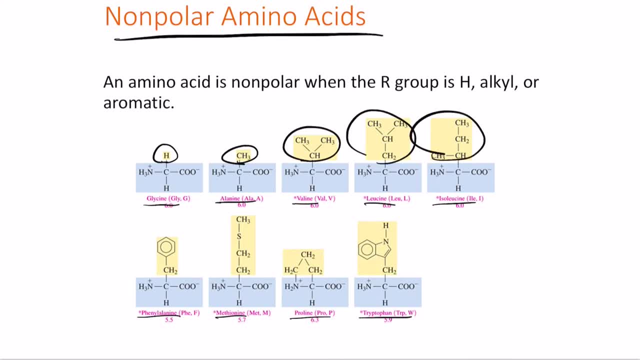 groups are either alkyl. so the first five of them here- glycine, alanine, valine, leucine and isoleucine- all contain a general structure of a alkyl group, so they have an alkyl or hydrogen. next you come to phenylalanine. this has aromatic structures. 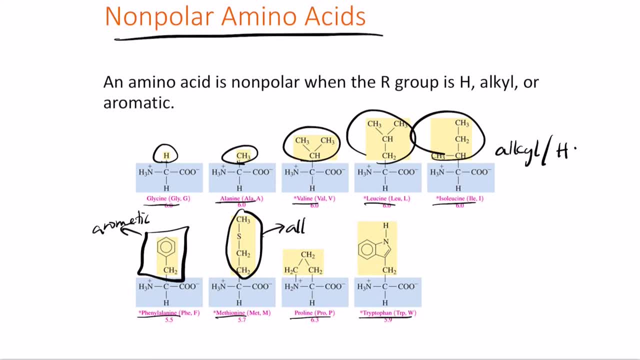 and you have methyl ionon. so this is alkyl. but it also has a sulfur in it, so it also has a sulfur group inside it, so it's a sulfide waste. so it's a sulfide group inside it, so it's a sulfide waste. 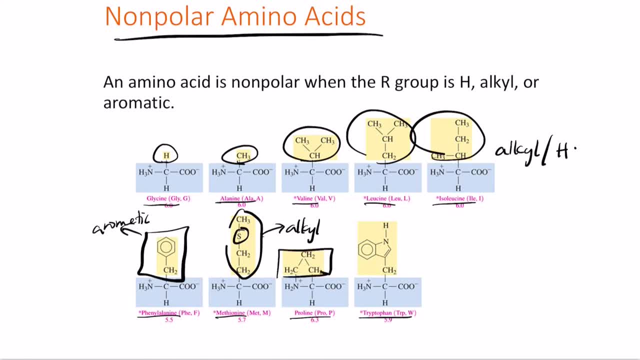 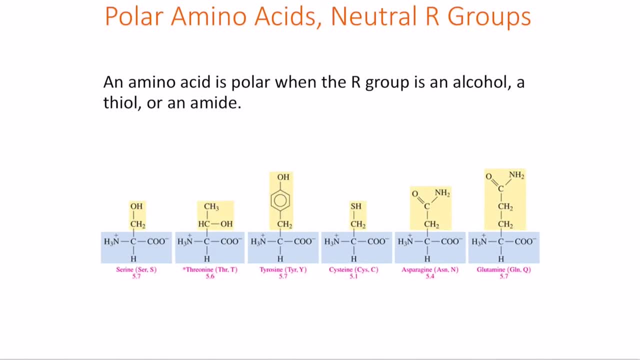 and this is the clorohydrate, and that is a group of macronutrients which are. that gives you an aromatic structure. and you have proline, which again has an alkyl group, but this is a cyclic alkyl group, and you have an aromatic structure on tryptophan. next, let's talk about polar amino. 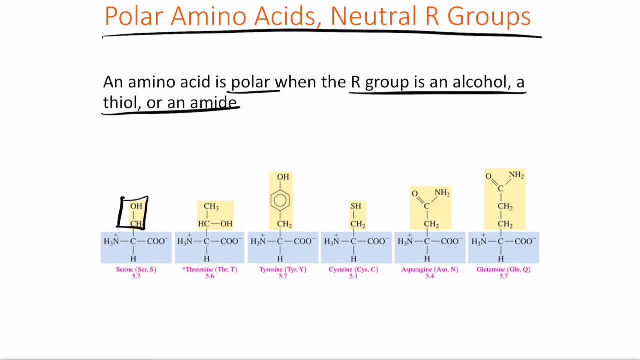 acids which are neutral, so polar amino acids. these are the ones that are polar, where the r group is an alcohol thiol or an amide. so serine is the first one with an alcohol group, with an aromatic alcohol group. you have cysteine with a sulfur thiol and you have aspergine with 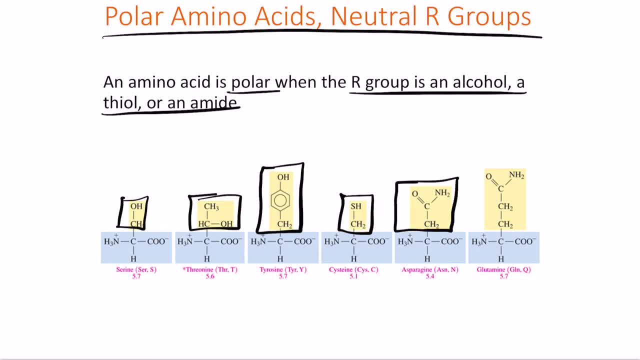 also an amine group, but here it's an amide. so notice that it is a c double bond, o, nh2, which is an amide. again, you have an amide group here. so there are two amides. these two are amide structures- aspergine and glutamine. and cysteine is the one that contains a thiol, tyrosine is the 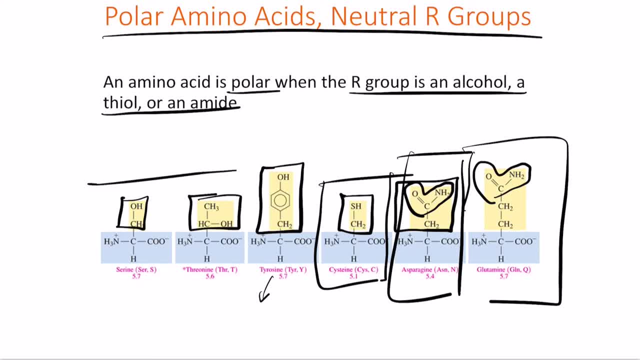 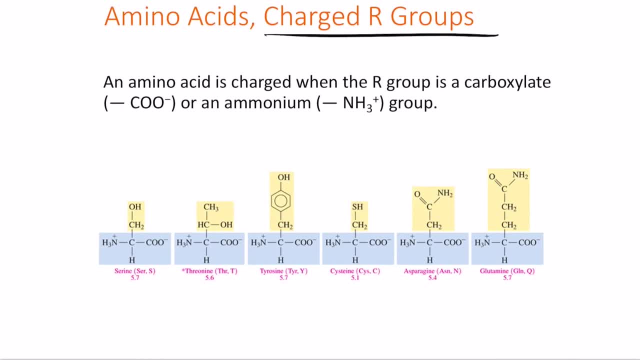 one that contains an aromatic alcohol. so the rest of them are alcohol groups. so this is how we can classify the polar amino acids, which are neutral. next let's come to the charged R groups, so an amino acid discharge, when the R group is a carboxylate or an ammonium ion group, so which? 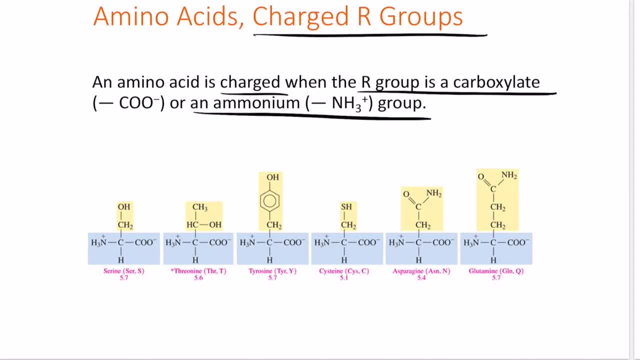 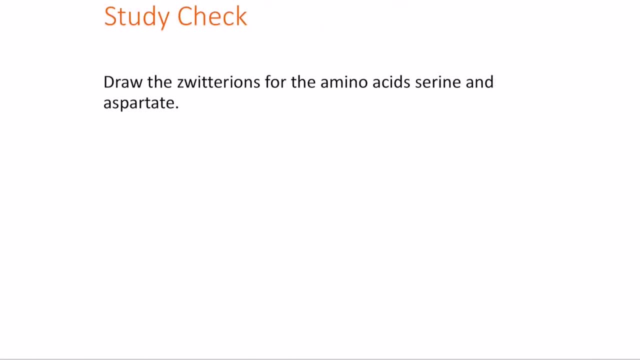 means that here. so we can take the same exact amino acids and let's consider how to draw the zwitter: 0, 0 ions of amino acids, serine and aspartate. let's take serine structure. so serine structure involves the entire structure. but in place of what we do here is we: 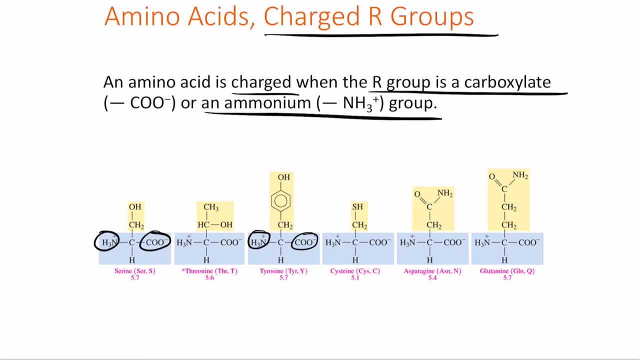 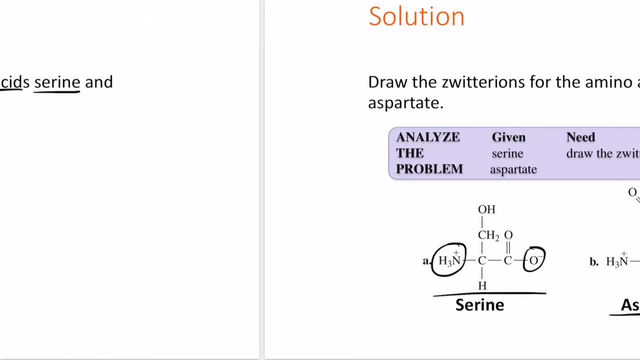 basically take in the NH3COOH and write down the structure, basically make sure that one is positive and the other is negative. if you take aspartate aspartate, if you take aspart aspergine, you notice that structure here: aspartate. 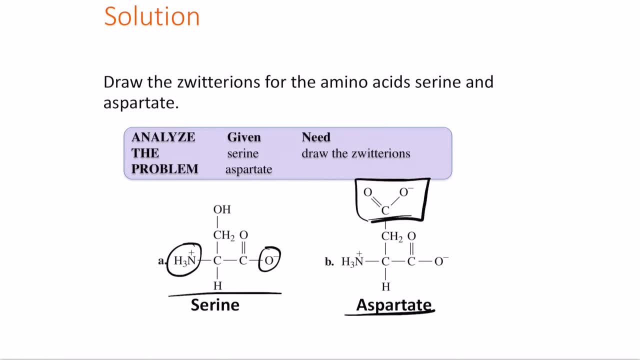 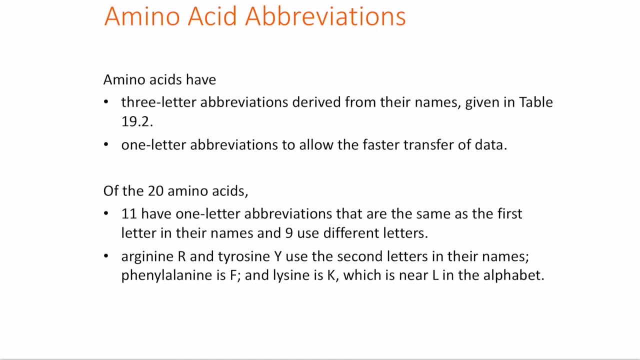 basically contains the exact same structure, but with the COO minus attached to it. so there are two COO minus acid and then one NH to prove. so this is these vitreionic structure of aspartate. now, how do you recognize this? amino acids and how do you name them? so these are generally given as 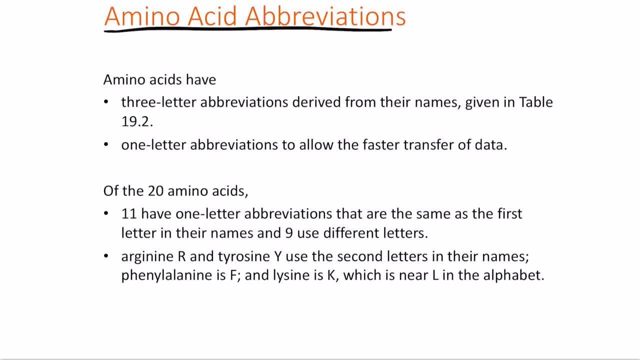 abbreviations. the reason we give them abbreviations is because it's easy to understand the structures. so we use a three letter of abbreviation that is generally derived from their names, and we also use one letter abbreviations okay to allow faster transfer of data as we write down the structures. so of the 20 amino acids we have, 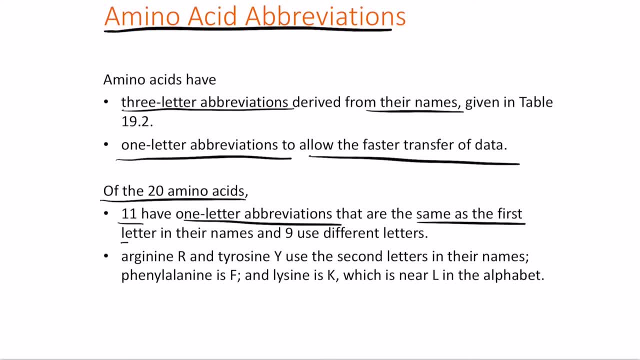 11 of them that have one letter abbreviations that are same as the first letter and in their names, and nine use different letters. for example, arginine uses r because aspartame can be written as the same a, so we use r to start with the structure. tyrosine has y because it's a second. 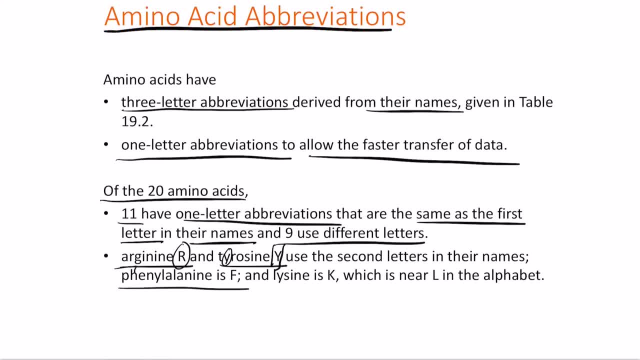 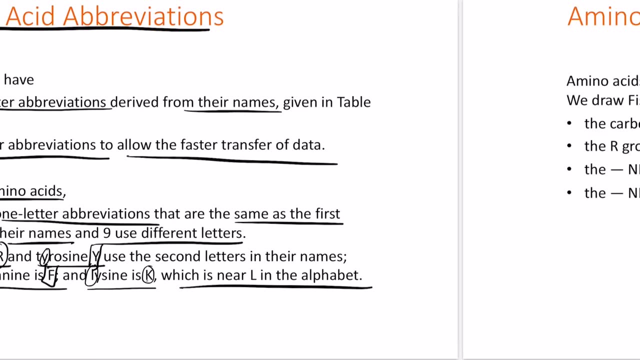 letter. so next we have phenylalanine, because the ph smells, you know, sounds like f. that's why we use f here. lysine: we use k because in the letter of the alphabet k is after, l is after, so k is after l. so that's the reason why, which is nearest to the l in the alphabet. now there are isomers as well. 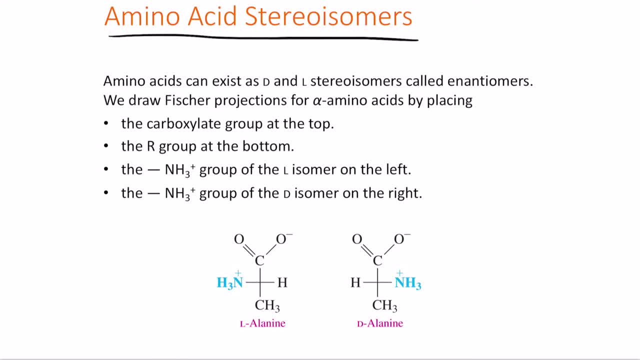 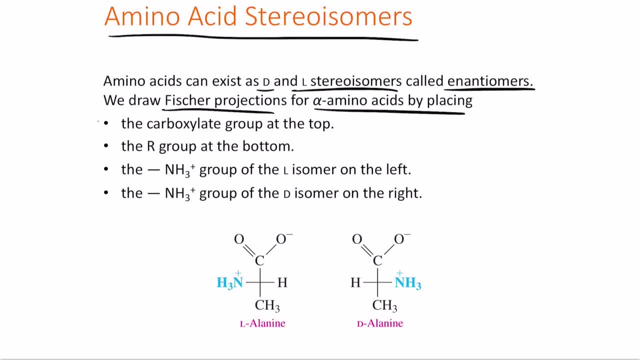 either. so how do you draw the fischer projections? number one: always place the carboxylate group on the top, the r group at the bottom and the nh3 group. if it is on the left side, we call it the l isomer. if it's on the right side, we call it the d isomer. so make sure that the carboxylate is on. 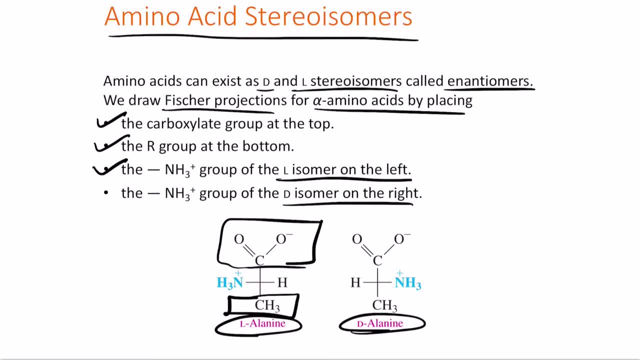 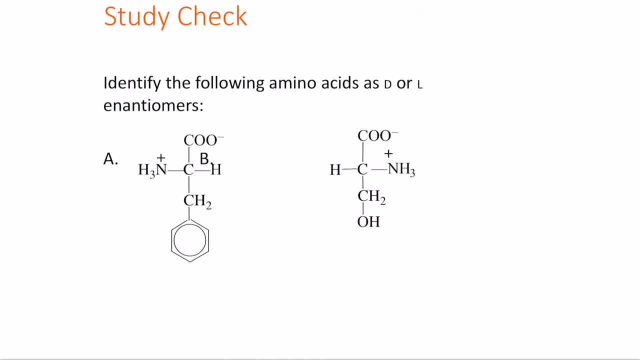 the top and the r group is on bottom, and once you keep it that way, if the nh3 is on the left side, we call it l, if it's on the right side, we call it d. so pause the video right here and try to name this structure. 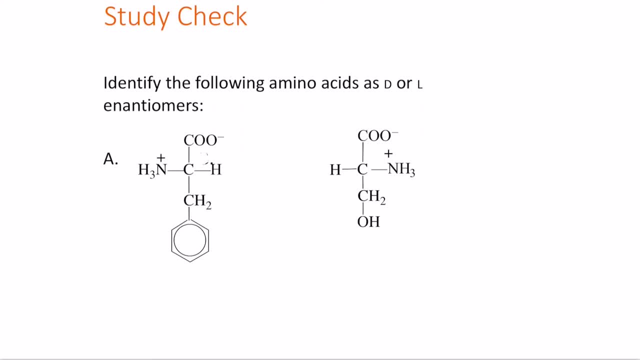 so notice that here the coo is on the top and the group is on the r. group is on the bottom. here also, coo is on the top, r group is on the bottom. here nh3 is on the left side, here nh3 is on the right. 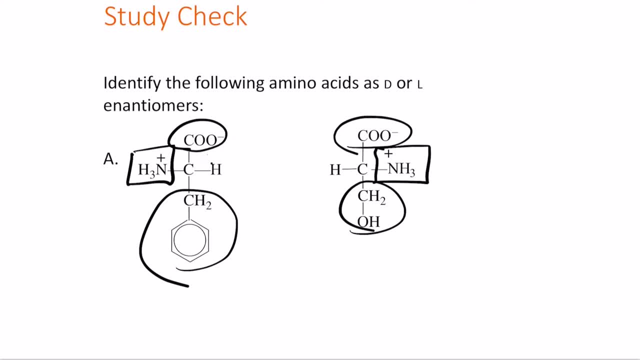 side. now, first thing we need to do is compare it with all the alcohols that you have seen. notice that this is the one that contains a phenyl group and a ch2. this is the one that contains a phenylalanine. i'm sorry, this is phenylalanine. 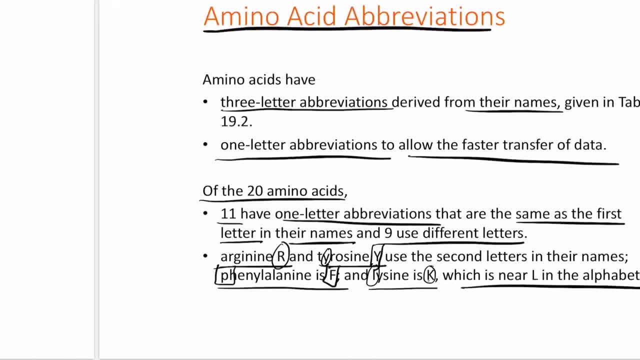 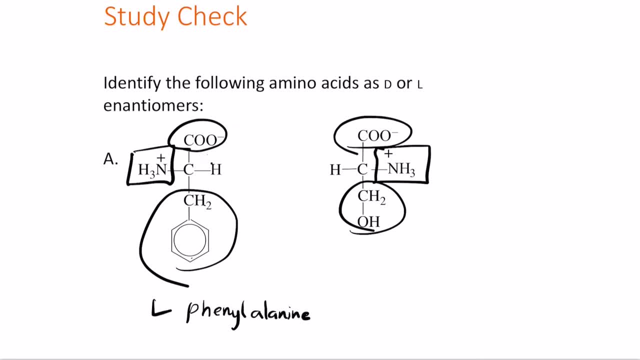 so phenylalanine and this is on the left side. so we write l phenylalanine and you have ch2oh attach it to it. so if you remember the original structure of ch2oh, notice that the structure is for serine. so this is: nh3 is on the top and the group is on the left side, so we write l phenylalanine. 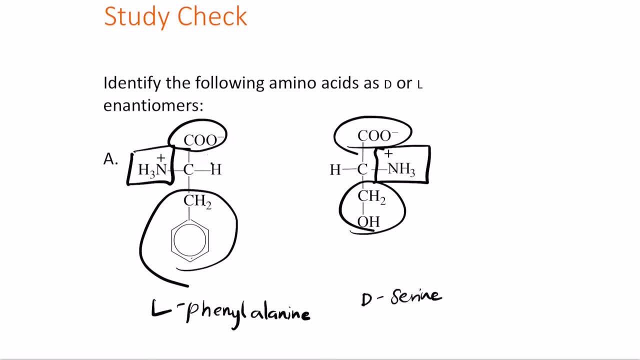 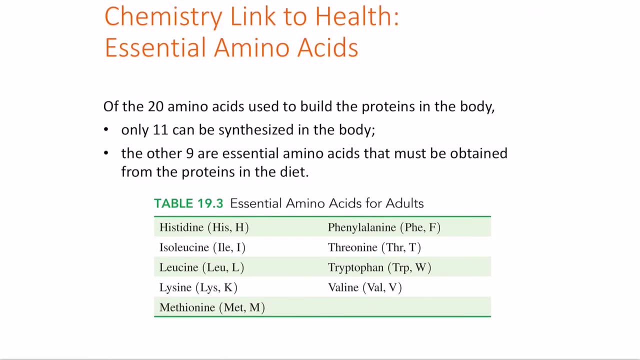 nh3 is on the right side, so we write d serine. this is how we can name the structures based on the positioning of the nh3 group. now let's talk about essential amino acids. so there are 20 amino acids in total that are used to build proteins in the body. out of them, only 11 can be synthesized. 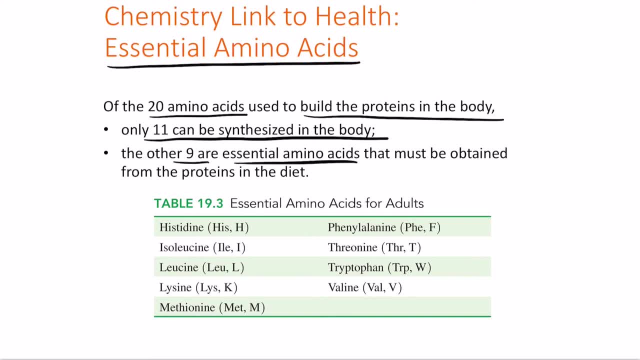 in your own body. the other nine are the essential amino acids that you have to get from proteins in the diet. so these are the essential ones: histidine, leucine, leucine, lysine, methionine, phenylalanine, threonine, tryptophan and valine. so these are the 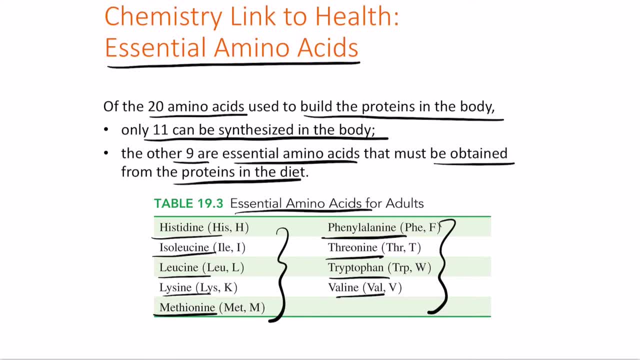 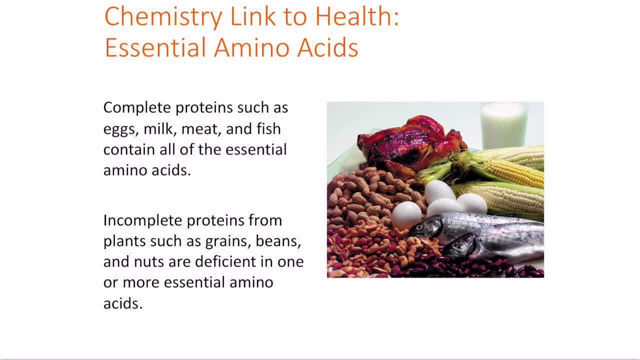 nine amino acids that are called the essential amino acids. the reason we call them essential is because these are not produced in your own body and you need it from supplements. the supplement can be food. the supplement can be direct in ingestion of the protein themselves. now, complete proteins, then, such as eggs, milk, meat and fish, generally contain all of the essential amino. 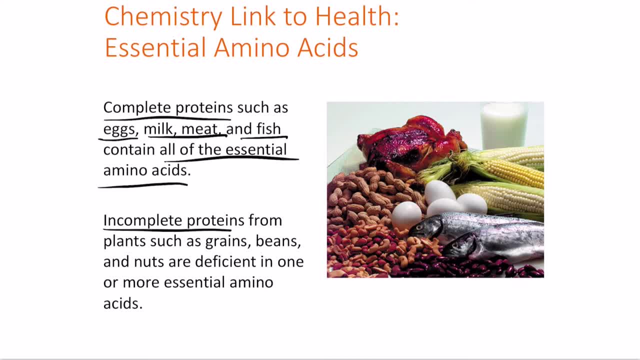 acids, but there are also what we call incomplete proteins. these are the ones that you get from grains, beans, nuts that are deficient in one or more essential amino acids. so that's the reason why meat has to be a part of your diet, and if you do not consume meat, you have to find a way to make. 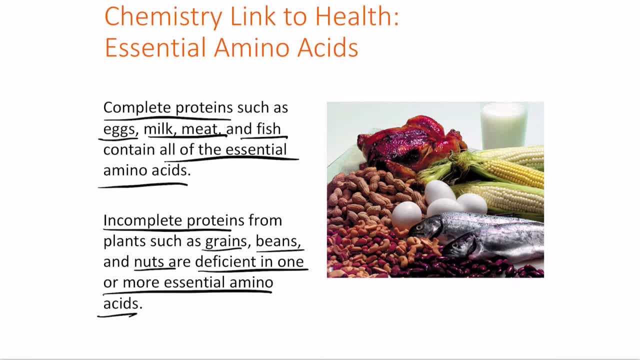 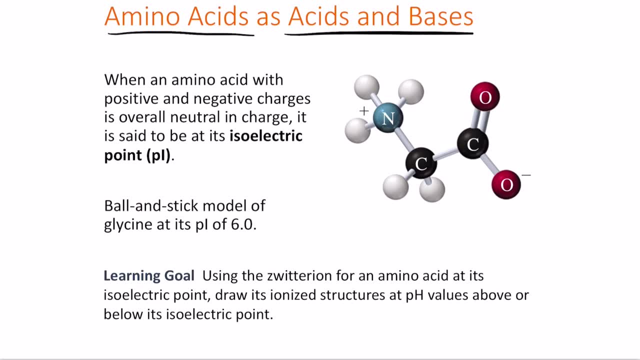 sure that you receive all the essential amino acids in the exact quantities that are required by your body. next, let's talk about amino acids as acids and bases. so we said that an amino acid exists as a ion at physiological ph and it can act as a base on an acid, and it stays neutral at isoelectronic. 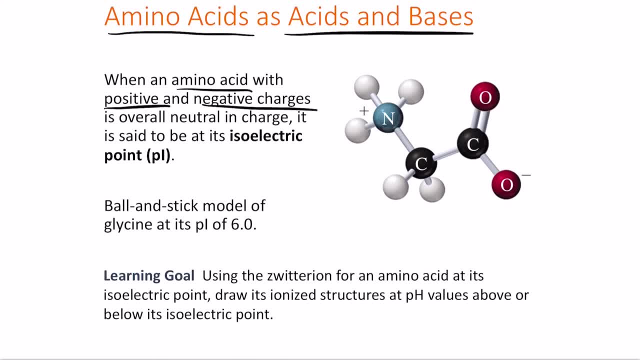 point. so when an amino acid with both positive and negative charges is overall neutral in charge, we call that, we said, to be at isoelectronic point. so this structure that you see here is a common structure of an isoelectronic point of a protein. so this is the pi of glycine at 6.0. now, 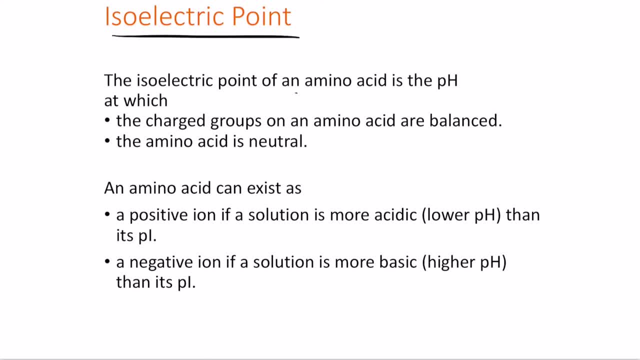 what is the isoelectronic point of a ph? so an isoelectronic point of an amino acid is basically the ph at which the charge groups on the amino acid are balance and the amino acid is neutral. now amino acid can exist as a positive ion if the solution is acidic, which means it has 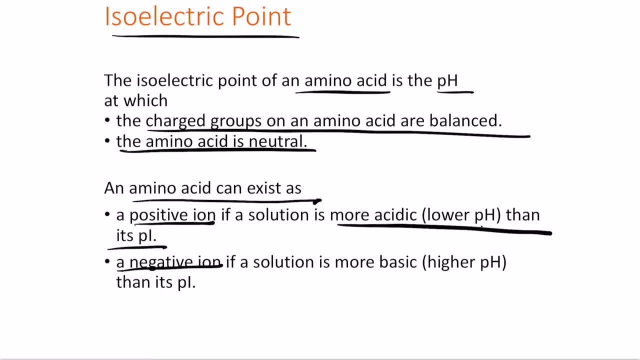 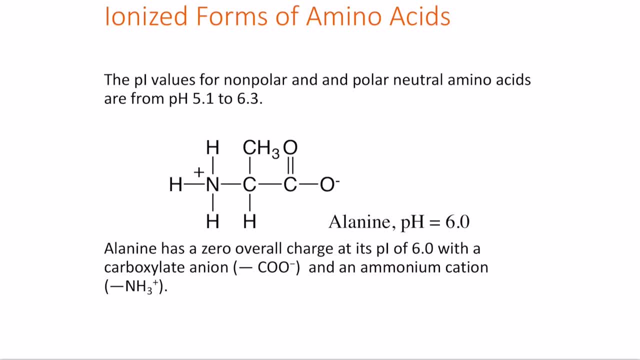 lower ph than its pi, it can exist as a negative ion. if the solution is more basic is a higher ph than its pi. so what about the amine ionized form of these acids? so the piικό acid must? values of nonpolar and polar neutral amino acids generally range from 5.1 to 6.3.. Now if you take 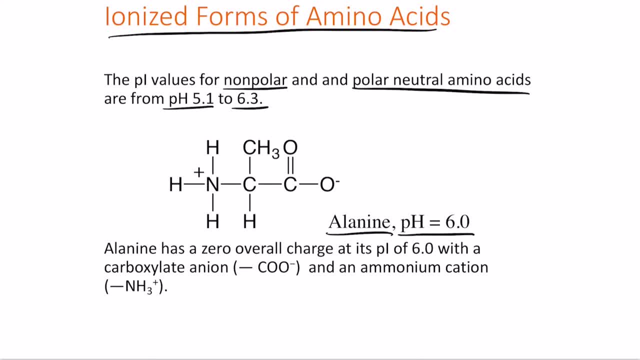 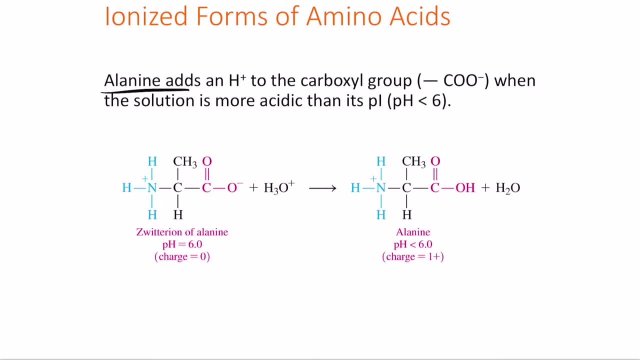 alanine at its pH of 6.0. it has a zero overall charge at its PI of 6.0, with the carboxylate ion which being negative and the ammonium cation which becomes positive. Now alanine basically adds a H plus to the carboxylate group when it is becoming more acidic, so creating an alanine which 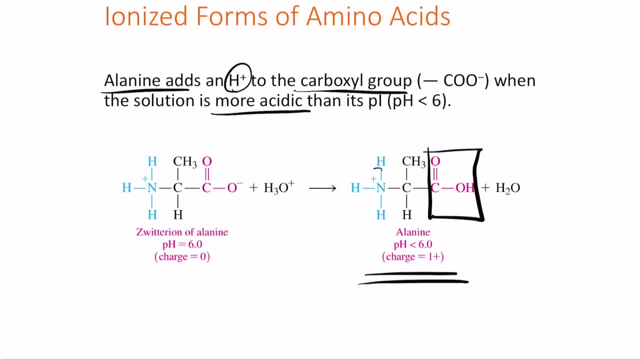 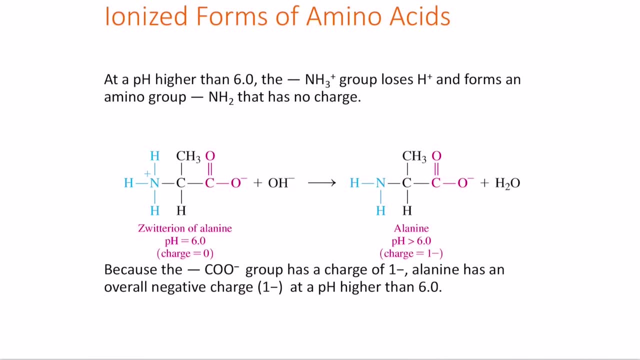 has an entire COOH group attached, which results in the formation of a positive charge, because the solution becomes becomes more acidic. Now, if the solution has a higher pH than 6.0, then the NH3 group will lose a H plus ion and forms an amino group, so which results in the 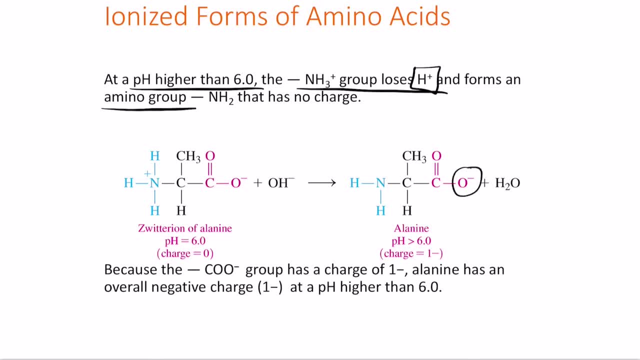 formation of a negatively charged alanine ion. So because both COO group has a negative charge and alanine ion, it becomes more acidic. Now if the solution has a higher pH than 6.0, then the alanine has an overall negative charge. will have a higher negative charge at a pH greater than 6.2. 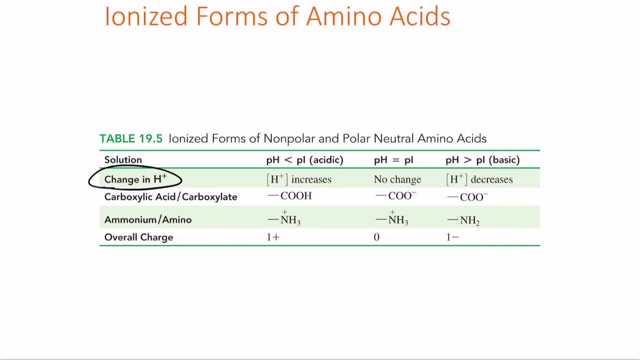 Now what happens when you change the change in H plus if the pH is less than PI, which means that if it is acidic, then the H plus concentration will increase. If pH is equal to PI, there is no change. Now, if pH is greater than PI, H plus will decrease In terms of carboxylate ion or 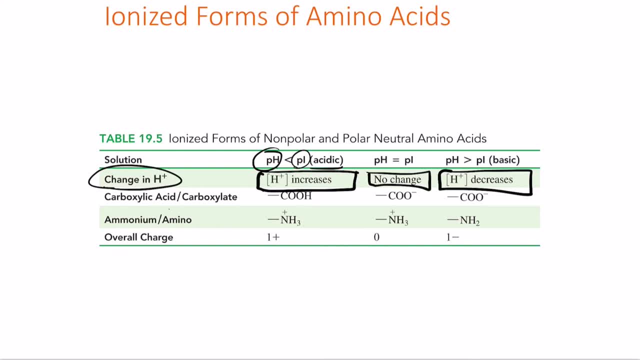 carboxylic acid. so when you have pH less than PI, it forms a COOH ion. When pH is greater than PI, it forms a COO minus ion, and pH equal to PI, it stays a COO minus. Now when, in terms of ammonium ion, when pH is greater than PI, it converts into NH2. but in the 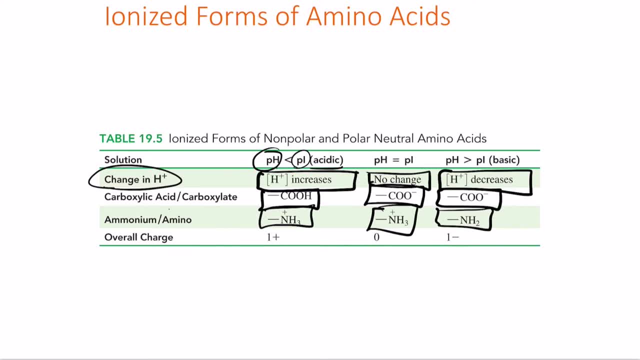 rest of the states it stays as NH3 plus. Now, when it is acidic, it becomes positively charged. when it is basic, it becomes negatively charged. For it to stay neutral, the pH should be nearly equal to PI. So these are the ionized forms of pH. Now, if the solution has a higher pH than 6.0, then the 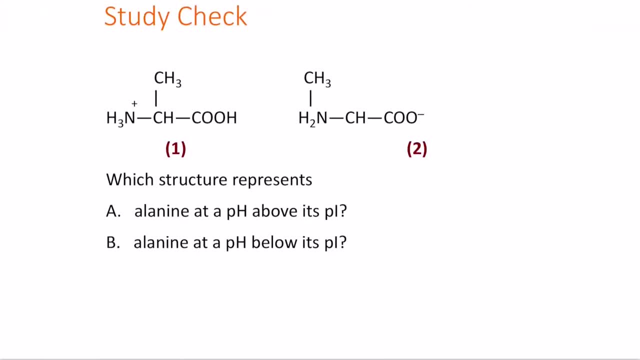 polar acidic and polar basic amino acids. So pause the video right here and try to solve this problem. They are basically asking you which structure represents alanine at a pH above its PI. So notice that when pH is greater than PI it means that this is more acidic, else more basic. So which means this time? 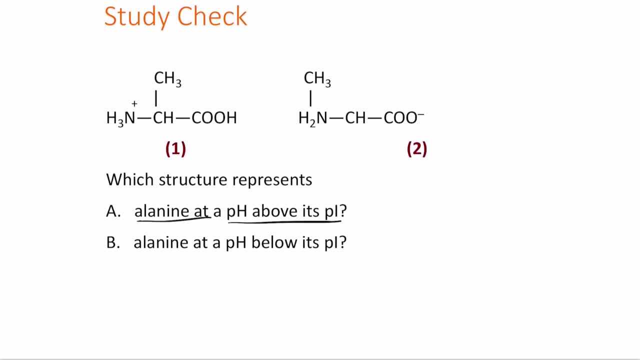 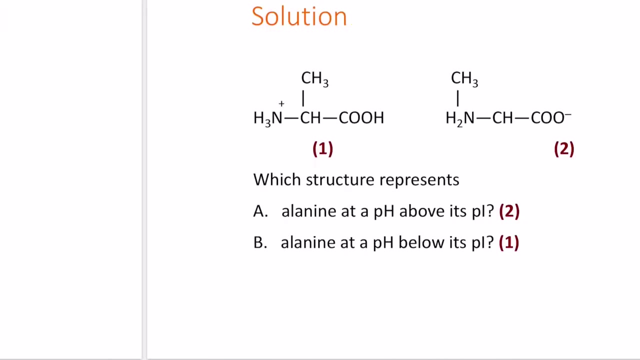 it has to have an NH3 group- sorry, NH2 group- with a COO minus existent. So this is the COO minus existent existent and it has an NH2 group. so which means this is the structure. so alanine below its PI will be number one. 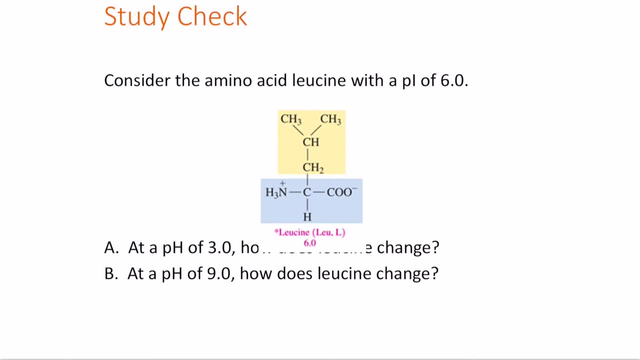 now consider the amino acid here. with a PI of 6.2, so at a pH of 3.2. so how does leucine change here? how will it change here? first thing that happens is that pH is less than PI. first thing that happens is that it adds COOH. so this: 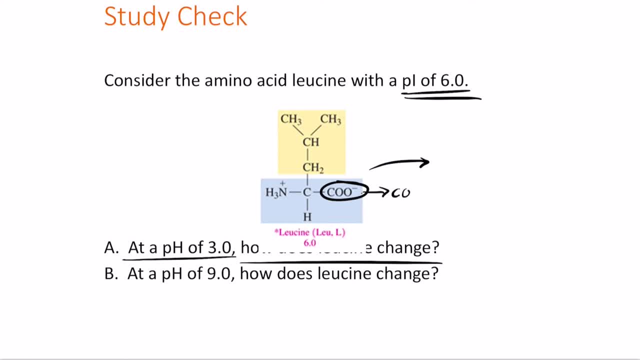 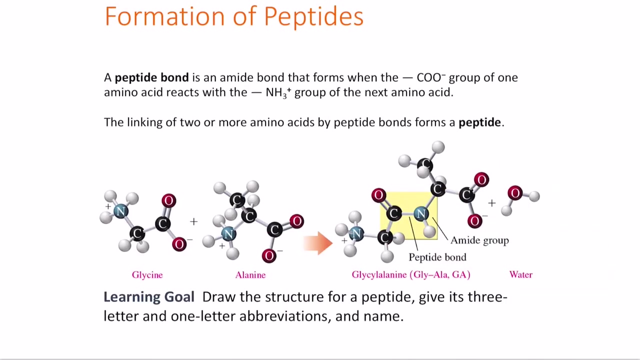 basically converts to the structure. this becomes COOH at a pH of 3, right? when pH is 3, this happens here. now, what a pH of 9? this becomes NH2, right? so this becomes NH2 at pH of 9. so this is how the leucine will change. next let's talk. 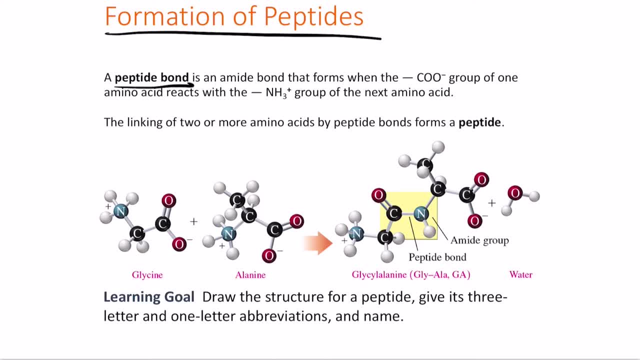 about peptides. so a peptide basically is a bond, is an amide bond, is an amide bond that forms between the COO group of one amino acid and the NH3 plus group of the next amino acid. so the combined form is what we call as a peptide bond. so 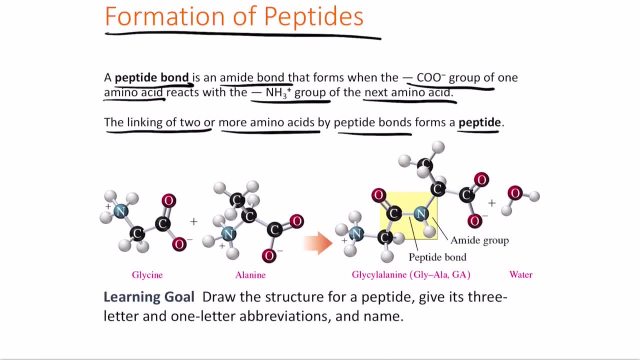 this basically links two or more amino acids by peptide bonds and this combination is called as a peptide. so what happens? let's say, for example, we are talking about glycine and alanine- when glycine, COO minus group bonds with the NH3 group, it creates the glycylalanine structure and the 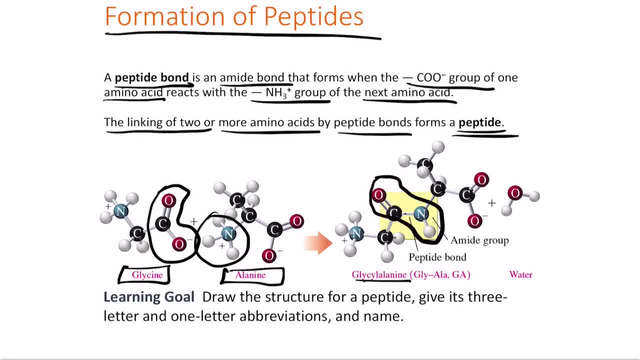 bond that forms here between CO- NH, so bond C, double bond, O bond NH here is called as the peptide bond. so this bond here is called as the peptide. so this peptide bond results in the removal of a H2O molecule. so two hydrogen's will go. 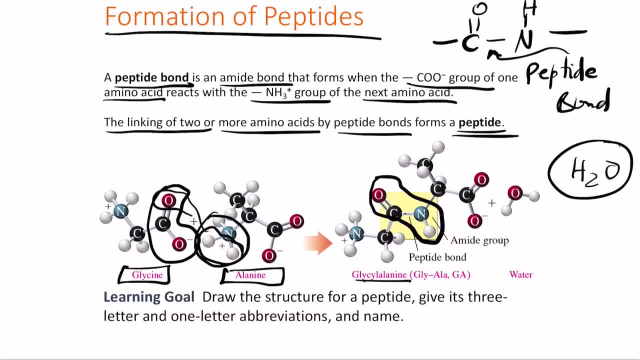 from the amino group. so two hydrogen's and one of the oxygen will move and the bond will form H2O and this is a dehydration reaction, which means that the there is a removal of water molecule from the structure and this creates the combined GA peptide. so this is 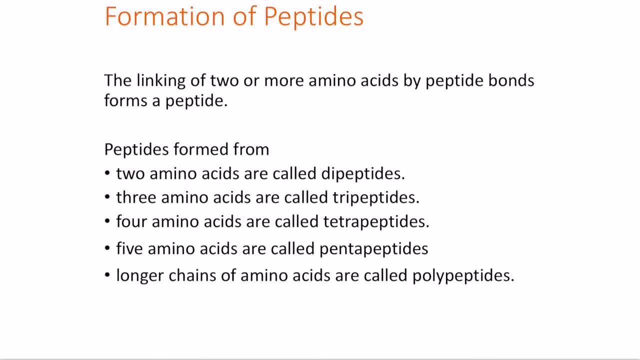 the structure that creates the form. now, the linking of two or more amino acids by peptide bonds clearly forms a peptide. so when peptides form from two amino acids, we call them dipeptides. when you have three amino acids- tripeptides- four amino acids- tetrapeptides and five amino 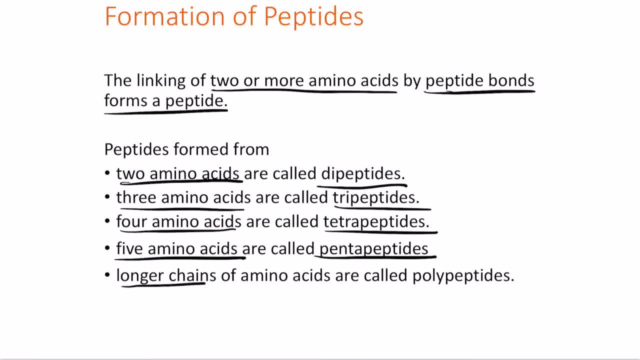 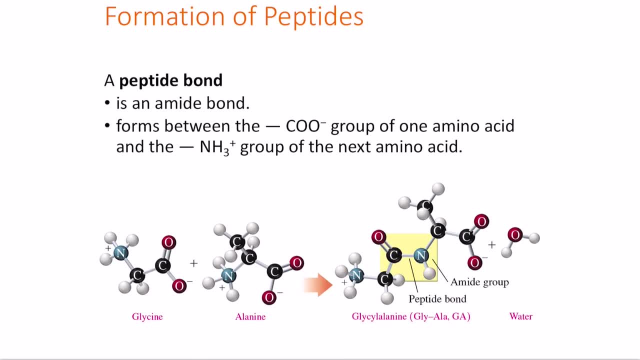 acids, pentapeptides anything longer than five. when you have longer chains of amino acids, we call them polypeptides. so remember this: names polypeptide. so what is a peptide bond? a peptide bond is basically an amide bond. it bonds when you have bond, COO bonds. 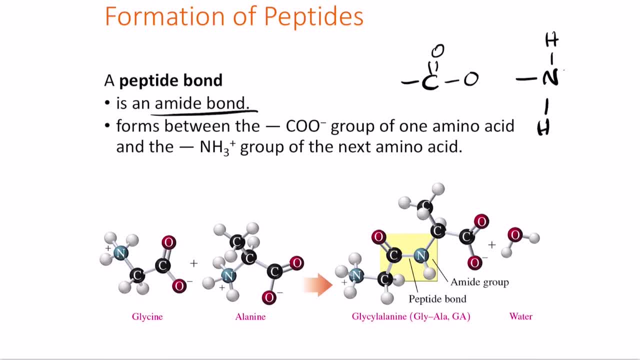 with the NH3 plus. so what happens here is that the two hydrogen's and one of the oxygen's will move out of the structure and the carbon will bond with the nitrogen, resulting in the formation of a C double bond, O- NH bond. so this here is an example of an peptide bond. 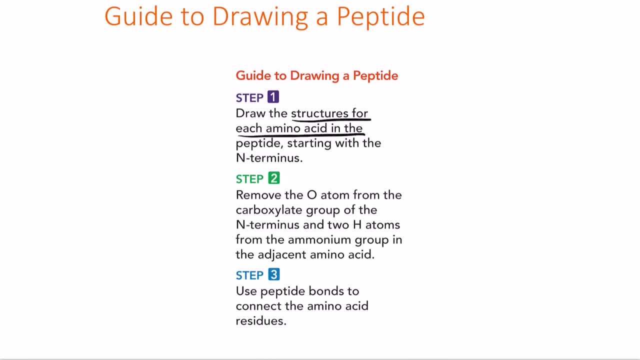 so how to draw the peptide bond? so first draw the structures of each of the amino acids in the peptide, starting with the N terminus, and step two, remove the oxygen atom from the carboxylate group and two hydrogen atoms from the ammonium ion in the adjacent amino acids and finally use. 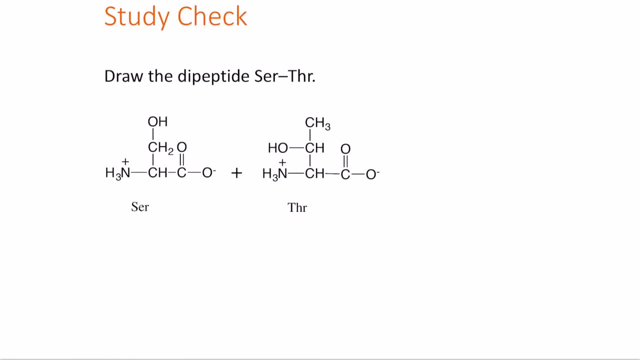 the peptide bonds to connect the amino acid residues. so, for example, here: what do we have to do first? so we have to remove this oxygen and we have to remove two hydrogen's from here, and both of them will combine and create H2O. now, whatever is left, write down the entire. 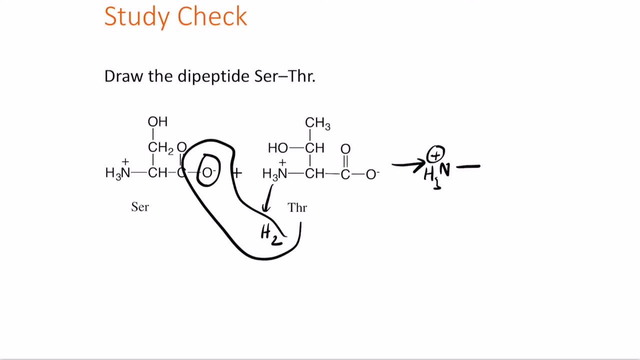 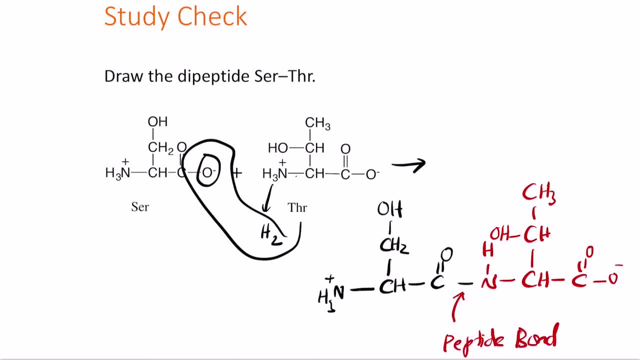 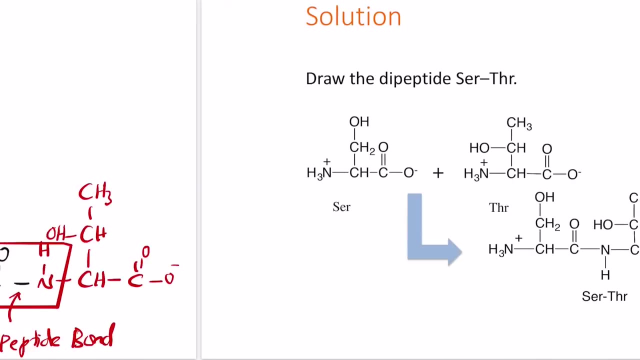 peptide bond. how do you know it's a peptide bond? so notice that it will have this: the natural C double bond O NH structure. so once you notice C double bond O NH, that is the peptide bond. so how do you name it? so this is serine, and 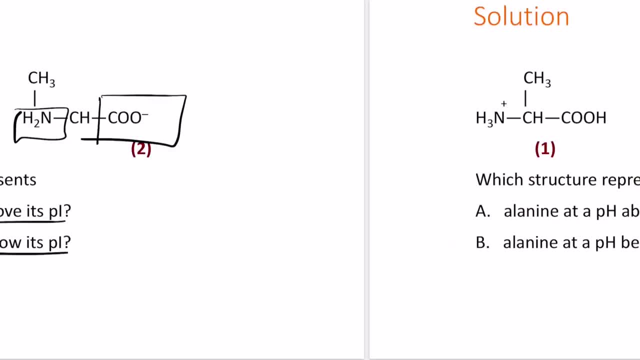 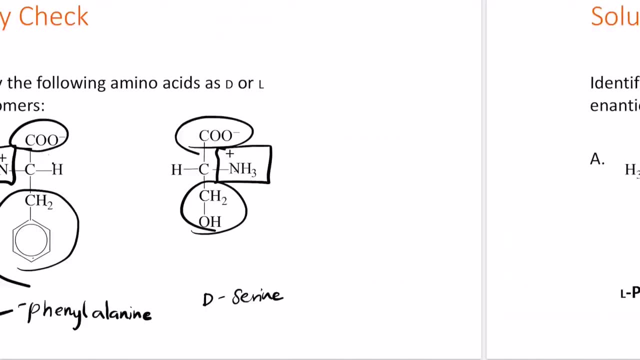 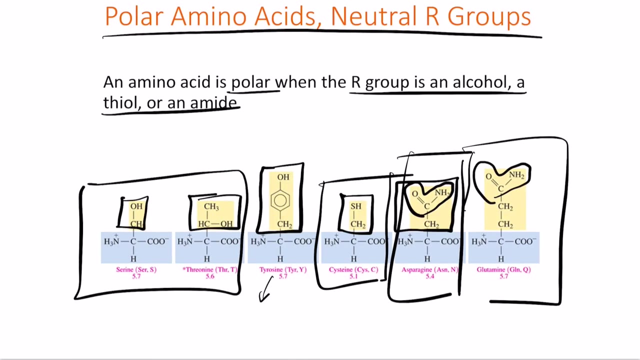 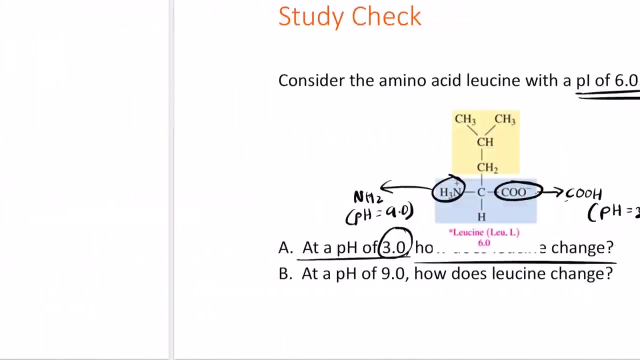 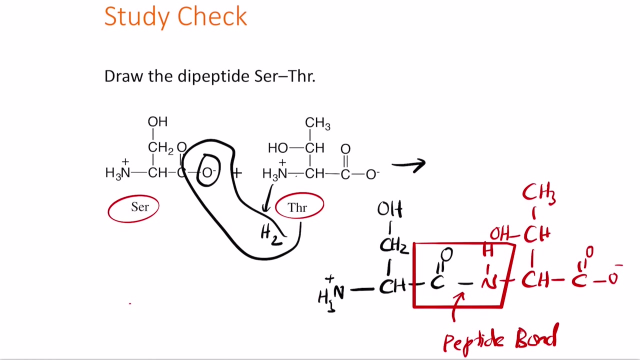 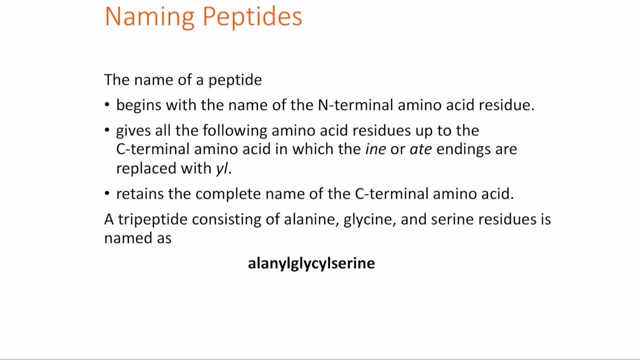 you have THR. I'm sorry, let me find the name for that particular structure. so 309, so this is serine and 309. 309, so we can write it as SER- THR, or the name will become serile, serine and THR. 309, so this is the combined dipeptide, so you can start naming more and more. 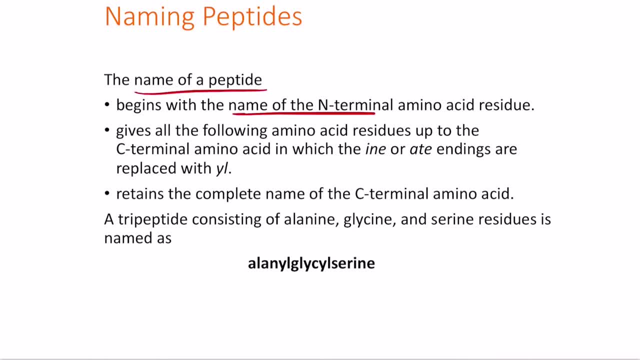 peptides as you go along. so the name of the peptide begins with the name of the n-terminus and the amino acid residue. so we start with the n-terminus, which is the north end of the structure, and gives all the following amino acid residues: 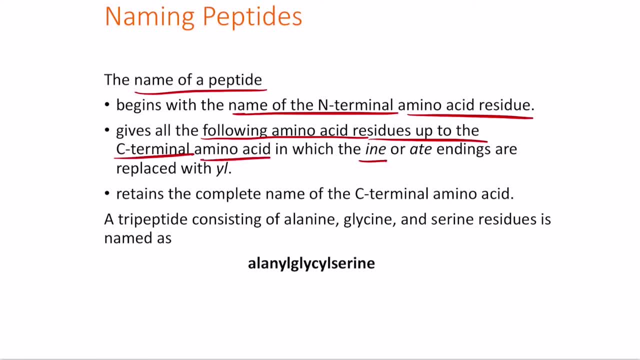 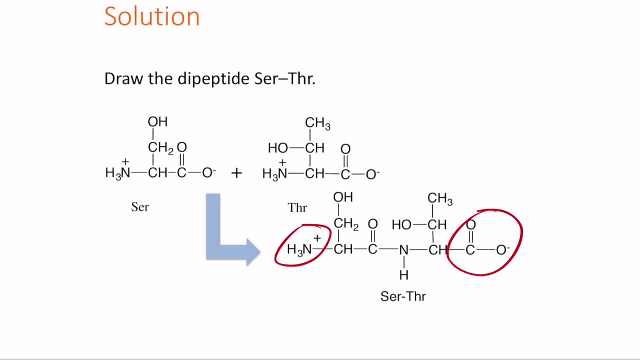 with the C terminal amino acid, with iron or eight. so the n-terminus is the one that contains the nitrogen and the C terminus is the one that contains the carboxylate ion. so we are always looking for the n-terminus here, the n-terminus to the C terminus. so the 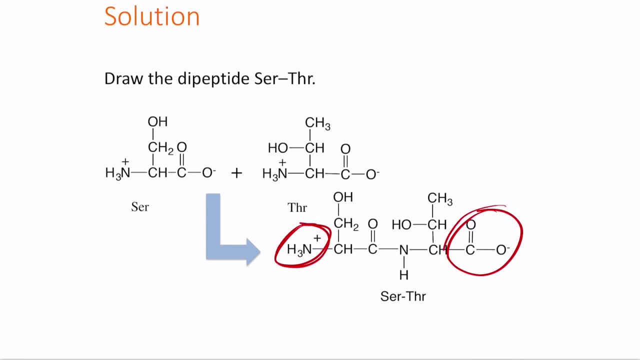 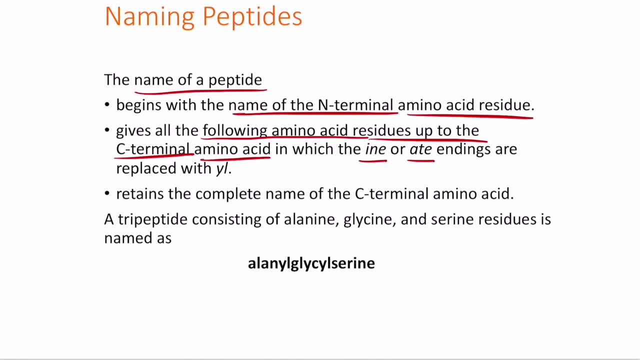 n-terminus. here is the end structure, so and the C terminus is the one that contains the C terminal structure. so we start naming the n-terminus side and the C terminus side will end with iron or eight, depending on, and we generally 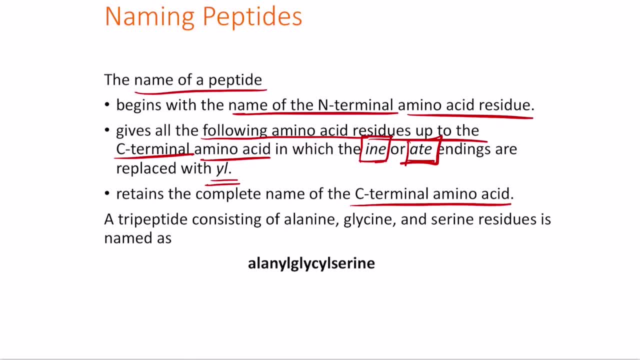 replace them with iron, and it retains the complete name of the C terminus: alkyl amino acid and the tripeptide of alanine, glycine and serine. here notice that alanine is the one that's going to bond with glycine, glycine is the one that 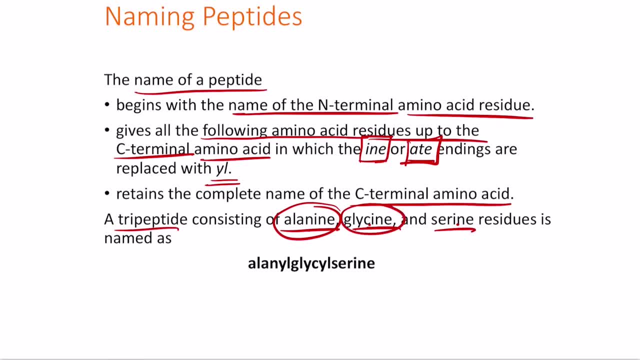 bonds with serine. so which means this one? these two will have the n-terminus and serine will have the C terminus. so serine will stay the same, but the one that has the n-terminus will become alanine glycine. so you have. 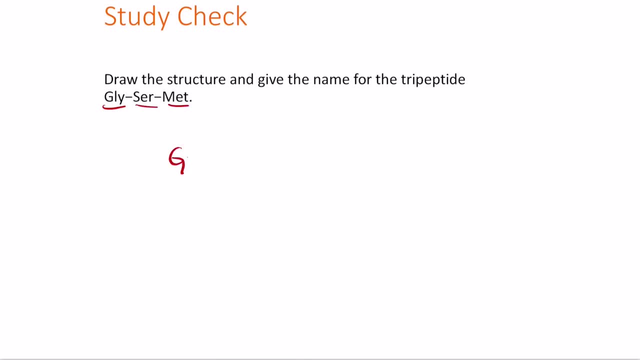 glycine, serine and methionine. so it becomes glycine, serine and methionine. so this is the name of the tripeptide and this is this structure of the tripeptide that you end up with. so GLY, ACR, MET or GSM. 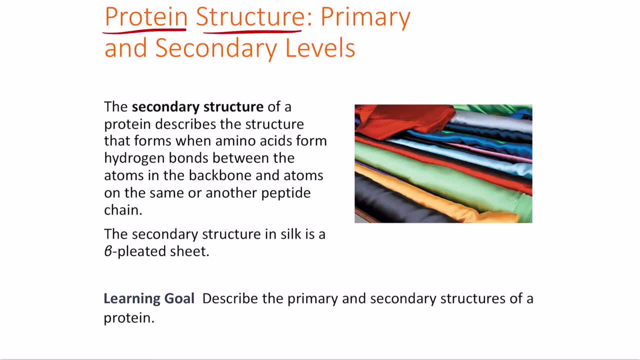 so let's talk about protein structure. let's start with the primary and secondary levels. the secondary structure of a protein is basically describes the structure that forms when amino acids form the hydrogen bonds between the atoms in the backbone and the atoms on the same or the other side of the peptide chain. so the secondary structure in silk is: 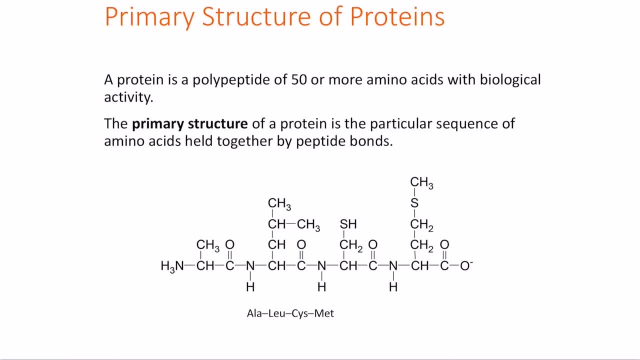 called as a beta-plated sheet, so we talked more about it as we go along. let's start with the primary structure of proteins. so a protein is a polypeptide of 50 or more amino acids. remember this part. this is very important. when do we name- not when we start naming- something as a protein? and 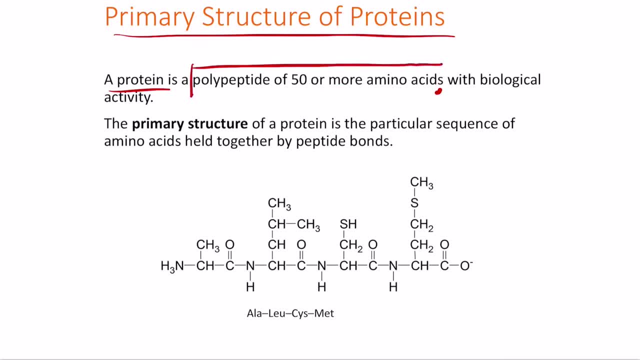 not a peptide- is when you have a polypeptide- 50 or more amino acids- that when we call a structure a protein. so notice that proteins are really large structures. that's the reason why, if you consider one amino acid is big, imagine a polypeptide of 50 amino acids. so this is the idea behind a protein. but what do we? what? 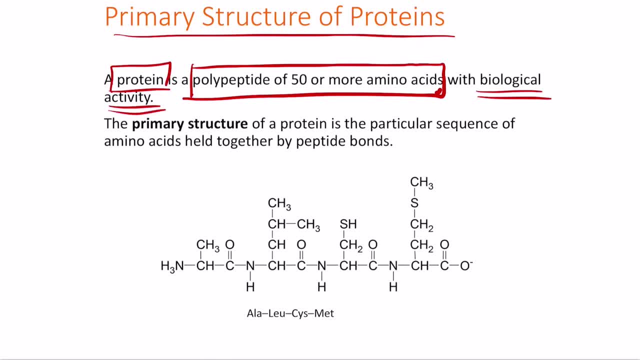 defines a protein separate is because of its biological activity. so anything that does not have a biological purpose is a peptide, and if the protein ends up becoming a biological activity, involved in the biological activity, we call it a protein. now, the primary structure of a protein is basically the particular sequence of the amino acids that held together, that are held together by 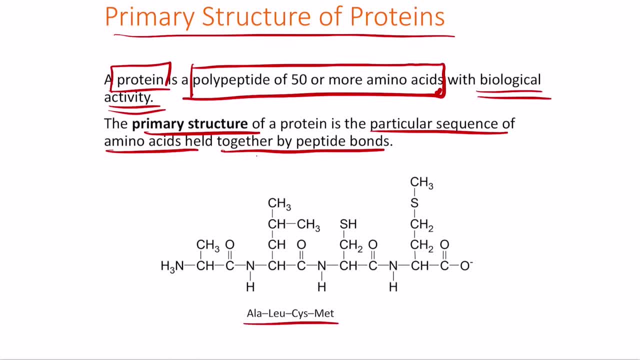 the peptide. so for example, here this is the peptide that has alanine, leucine, cysteine and methionine and all of these have. you have number one, two and three peptide bonds. so it is alanine, leucine, sissile methionine. so this is the 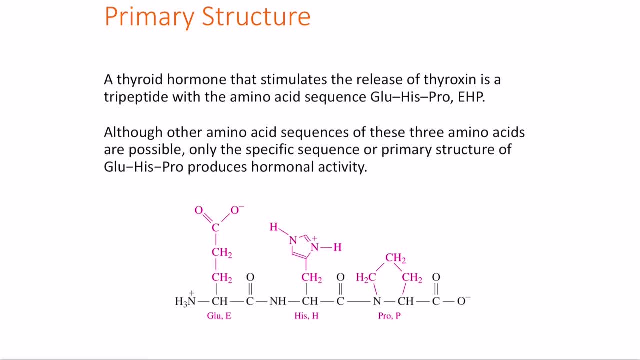 tetra peptide that we try here. so, for example, if you take the thyroid hormone, so the thyroid hormone that stimulates the release of thyroxine is a tripeptide with an amino acid sequence of glue, glu, his, pru or ehp, and although other amino acid sequences 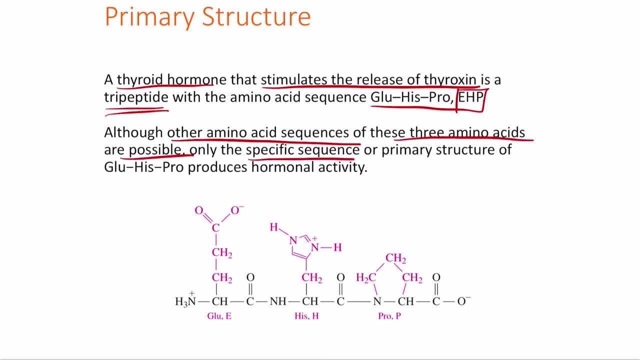 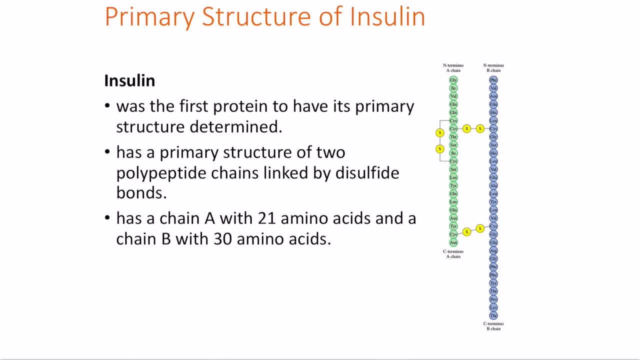 of these three amino acids are possible, but only specific sequence of the primary structure produces the hormonal activity. notice that you can have different, consecutive, different- you know combinations, but this is the particular sequence that results in the hormonal activity. that's why we call this a protein and not as a peptide. 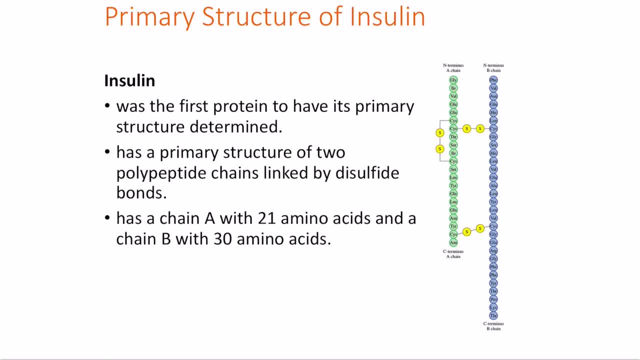 so this is the primary structure of insulin. notice the continuous chain of amino acids connected by sulfide bonds. you have sulfide bonds that are connecting these structures. so insulin was the first protein to have its primary structure determined and it has a primary structure of two peptide bond. 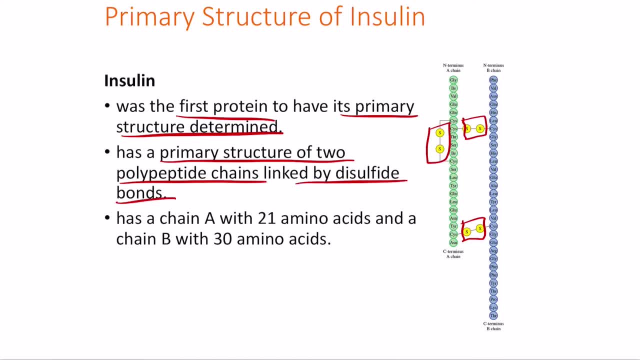 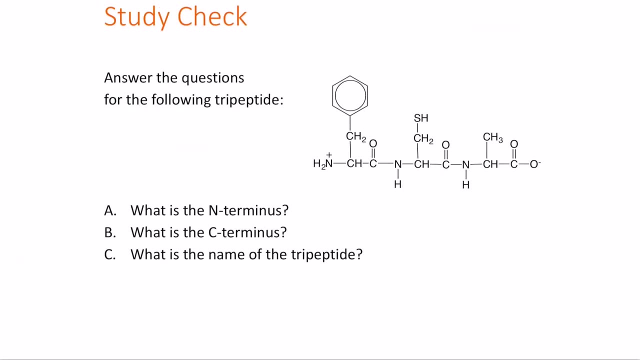 peptide chains linked by disulfide bonds and it has a chain A. so this is the first chain. so the chain A has 21 amino acids and the chain B here contains 30 amino acids and both are linked by disulfide bonds. so let's try and answer some questions for the tripeptide here, so they 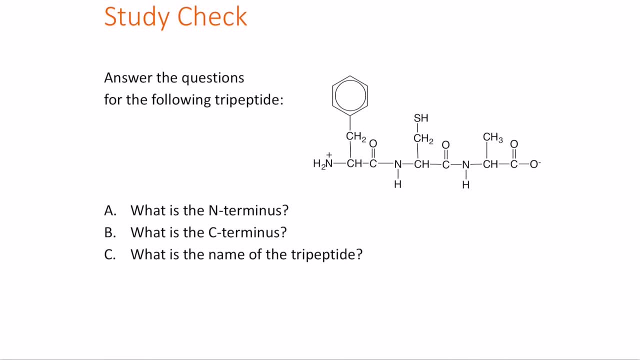 have given us a tripeptide and they're asking us: which is the? what is this? the N-terminus? so the N-terminus is this structure, the C-terminus is this structure. what is the name of the tripeptide? notice that first structure. 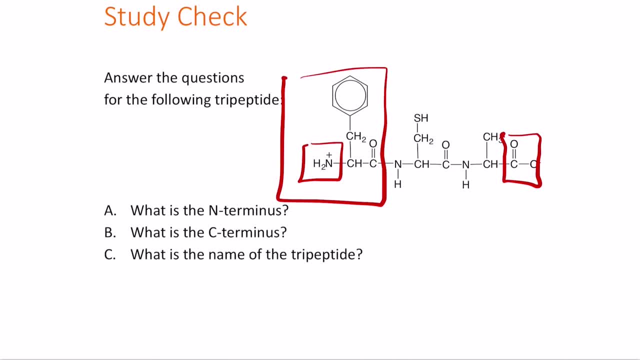 that we need to know is: what is this structure first? so we know that it's a phenylalanine one, and next you have this structure here. so next is this structure, and the last one is this structure. so we need to figure out each of these. 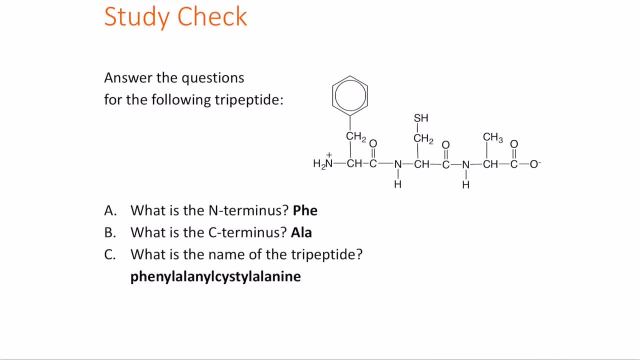 structures and what they know what, but they're named after. so the first structure is phenylene, the second structure is alanine and the last structure is cysteine. so the last structure is alanine. again, right, sorry, the last structure is alanine and the middle structure here is cysteine. so this is phenylalanine, this is. 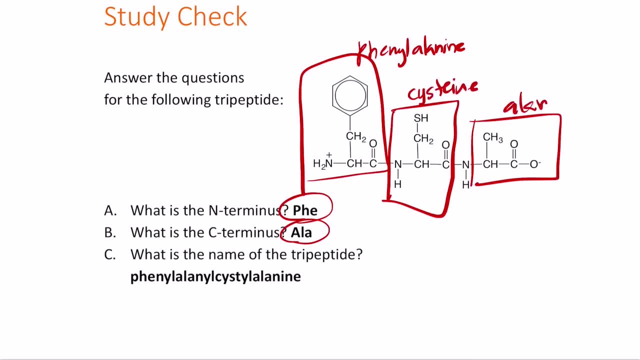 cysteine, this is alanine. so how would you name the structure? the N-terminus goes first. so if you have phenylalanine, so iron will go out, so it becomes alanine. so phenylalanine and you have cysteine becomes cysteine, alanine as the 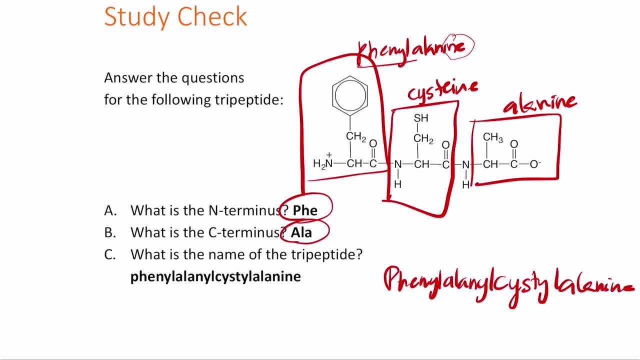 last structure, the C-terminus always has no change in this name. so this is the structure of the tripeptide that we have here. so we have a structure here and we the end terminus here is phenyl phenyl anodyne alanine, and you have alanine on the c terminals. 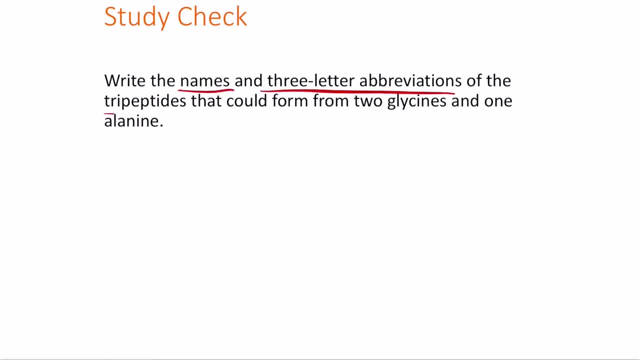 so they're asking us to write the names and the three letter abbreviations of tripeptides that could form from two glycines and one alanine. so you have two glycines and one alanine. so you have gly, gly, alanine. so gly, ala, gly and you have ala. 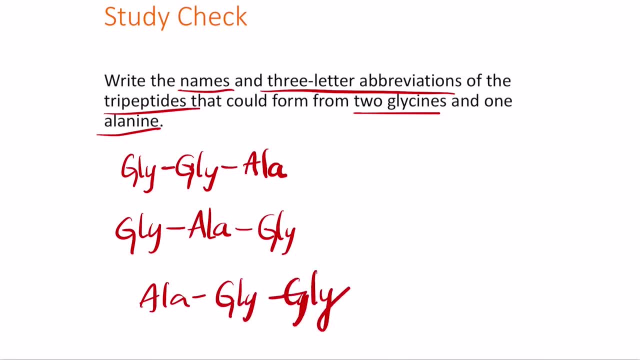 gy gy. so these are the three structures that you can form from two glycines and one alanine. so to pause the video right here, you already know the structures. use the slides from before or from the textbook. try to note down the right structure for glycine, glycine and alanine and write down the 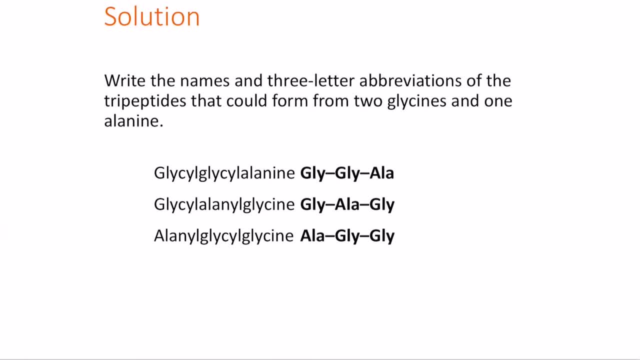 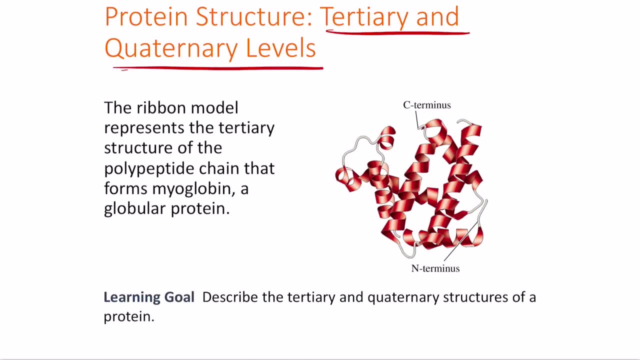 original tripeptides that are actually forming from this structure. next, let's talk about the tertiary and the quaternary levels. so the tertiary and quaternary walls are represent. we generally use them to represent the ribbon model, to represent the tertiary structure of a polypeptide chain. this is the one that forms either myoglobin, which is 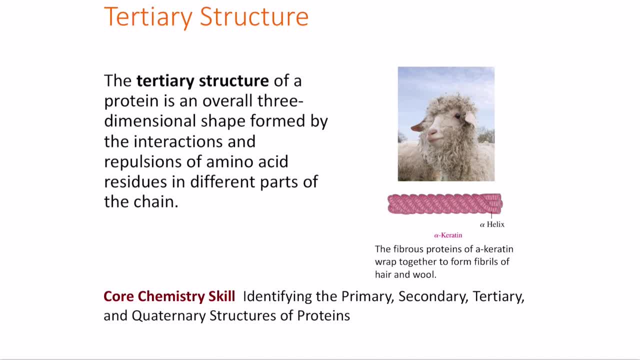 generally a globular protein. so let's start with the structure, the tertiary structure. the tertiary structure of a protein is the overall three-dimensional shape that it formed by the interactions and the repulsions of the amino acid residues and different parts of the chain. for example, the fibrous protein of alpha carotene creates an alpha carotene structure, which is 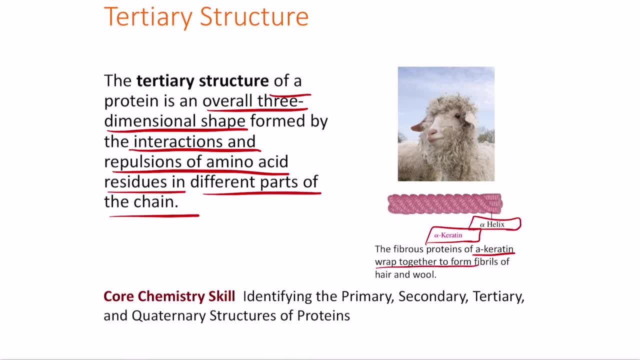 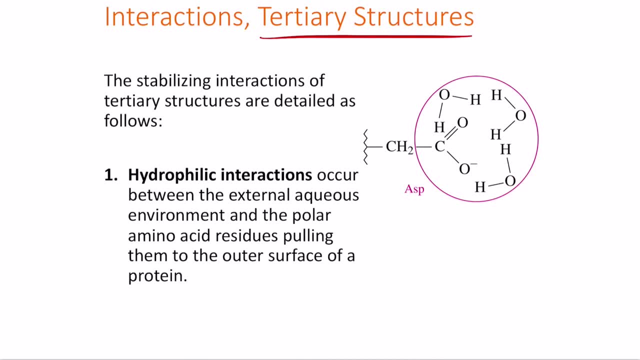 generally created by alpha helix structure which wraps together to form fibrils of hair and wool. now, when you take the tertiary structures- so the tertiary structures are generally includes by the stabilizing interactions of the tertiary structures that are detailed here. for example, you have one amino acid that are 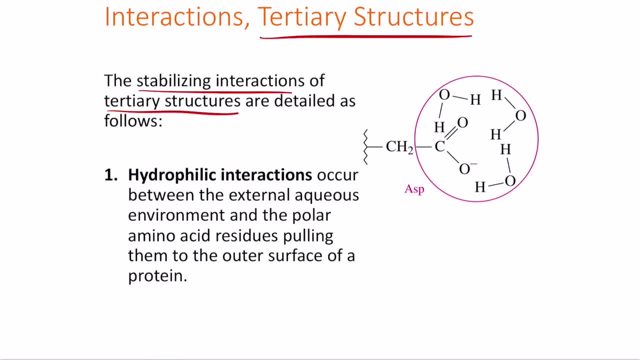 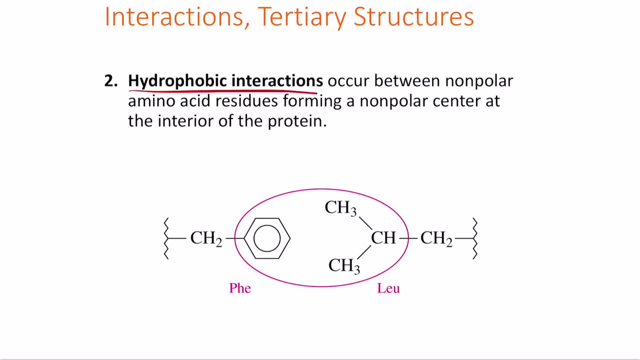 interacting with the different part structures of these structures here. one of them is hydrophilic interactions, which involves occurs when you have external aqueous environment and the polar amino acid residues pulling them to the outer surface of the protein. next, you have hydrophobic interactions that occur when you have nonpolar amino acid residues from 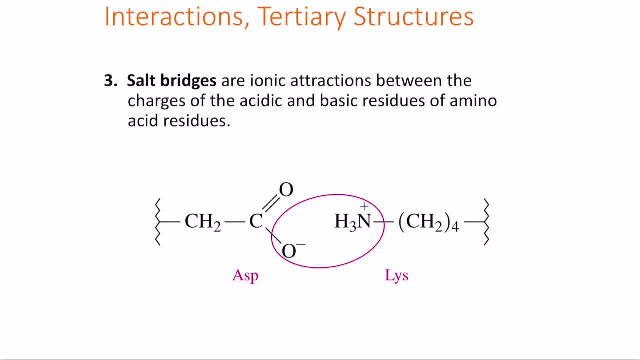 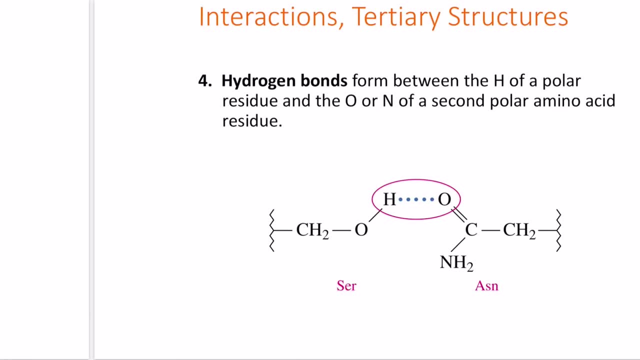 forming a nonpolar center at the interior of the protein. and you have salt bridges, that are ionic attractions between the charges of acidic and basic residues, of amino acid residues. and you have the final one, fourth one, which is the hydrogen bonds, which are the ones that bond between the hydrogens. 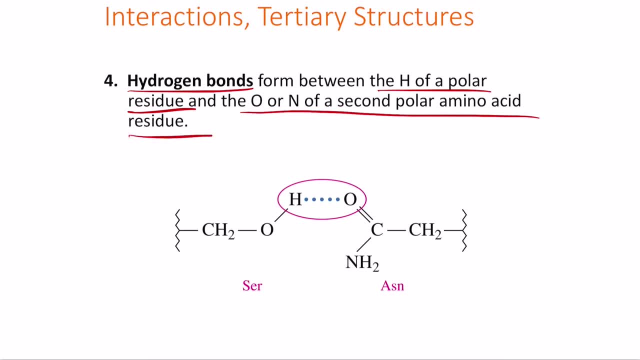 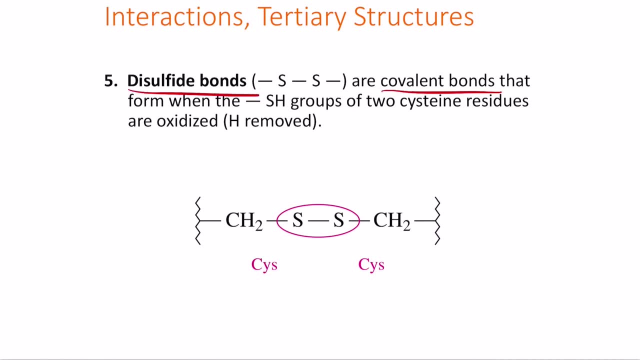 of polar residue and the oxygen and nitrogen of the or a nitrogen of the second polar amino acid residue. and the last one is the disulfide bond, which are the covalent bonds that form when you have sh group of two cysteine residues that are oxidized, removing the hydrogen, creating the disulfide bond. now, these interactions between 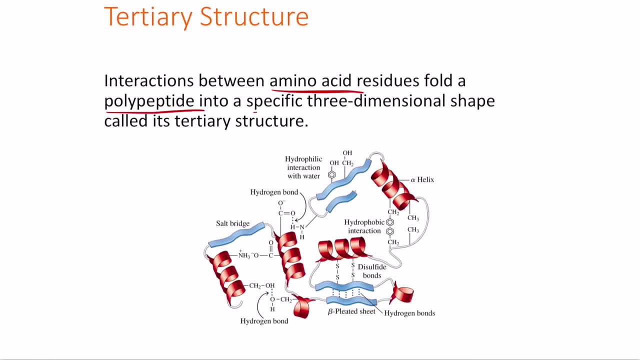 the amino acid residues fold the polypeptide into a specific three-dimensional structure, and that three-dimensional structure is what we call it tertiary structure. for example, you have alpha sheets, you have beta pleated sheets. sorry, you have alpha helixes and you have beta pleated. 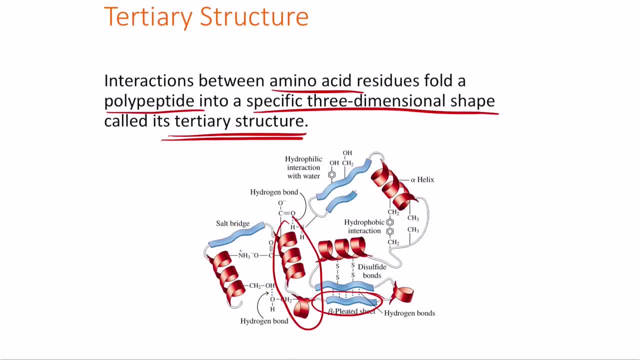 sheets. these are formed. these are bonded between the n terminus and the c terminus, are generally connected from one structure to the other structure, either by hydrogen bonds or disulfide bonds, or hydrophobic interactions or hydrophilic interactions, or hydrogen bonds or salt bridges. 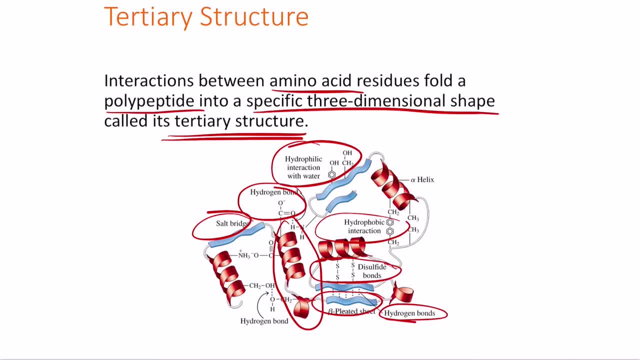 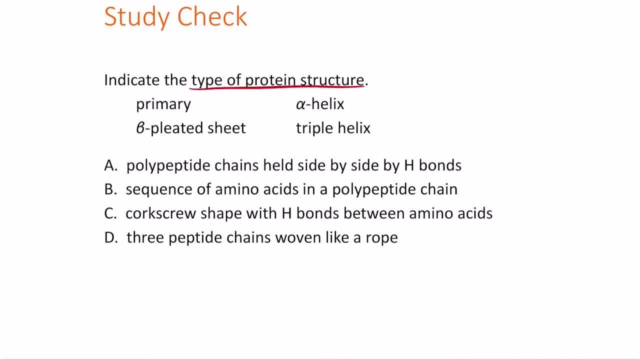 so this is how the entire structure comes together to form a tertiary structure now. so they're asking us to indicate the type of protein structure each of them is. number a is a polypeptide chain held side to side by hydrogen bonds. so whenever you have a side to side, 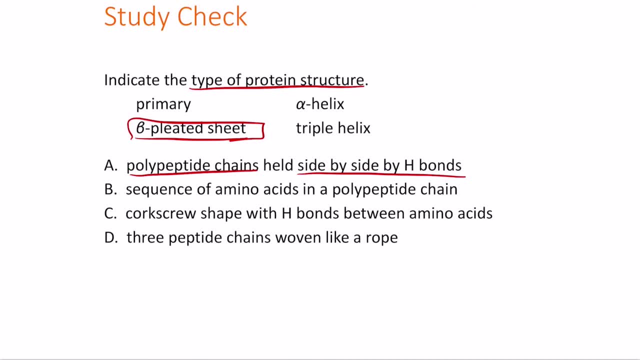 structure. it's a pleated sheet, remember this part. next you have a sequence of amino acids and a polypeptide chain. so, which is a primary structure, a corkscrew shape with hydrogen bonds between the amino acids. so a corkscrew shape is an alpha helix: three peptide chains woven like a rope. so that's a. 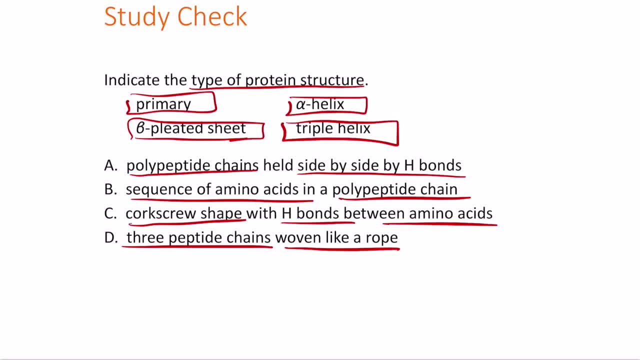 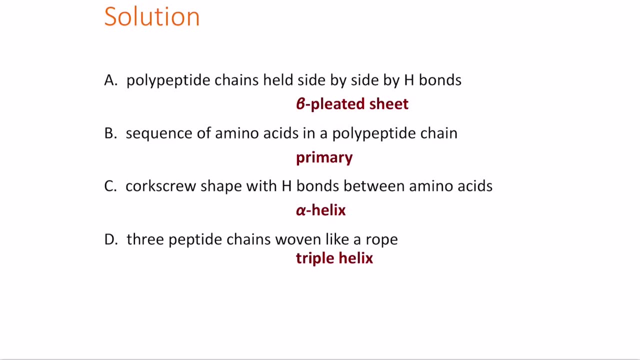 triple helix, so one structure covering over the other structure. so this is how the interactions generally happen inside the structures here. so, and this is how we can name the structures. so now let's talk about globular proteins. so let's start with the first one: myoglobin, so globular. 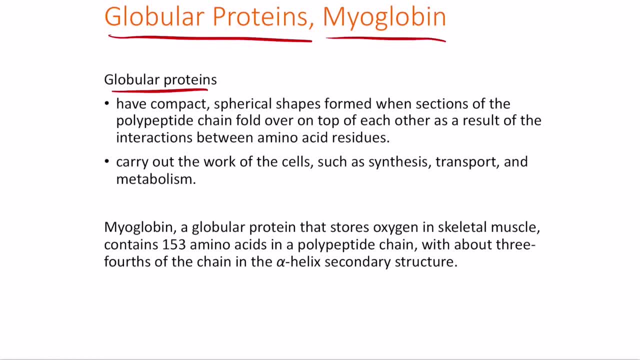 proteins are generally the ones that are the largest of all the proteins. these are compact spherical shapes formed when you have sections of the polypeptide chain fold over the top of each other as a result of interactions between the amino acid residues. and these are the ones. 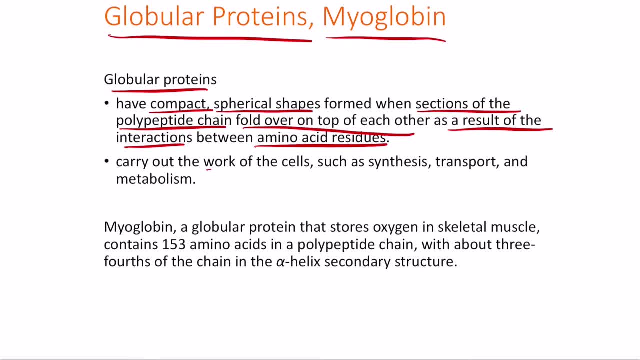 that are responsible to carry out the work of the amino acid chain. so these are the ones that are responsible to carry out the work of the cells, such as synthesis, transport and metabolism. for example, you have myoglobin, which is a globular protein that stores oxygen in the skeletal muscle. 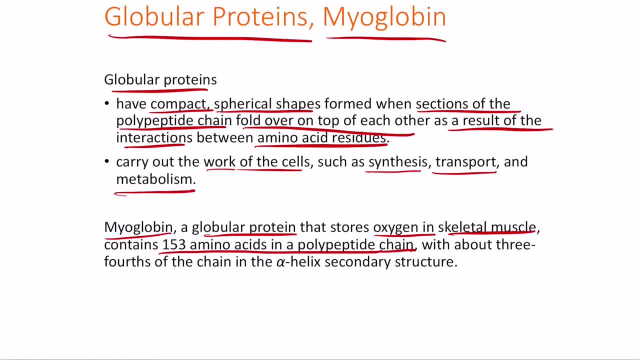 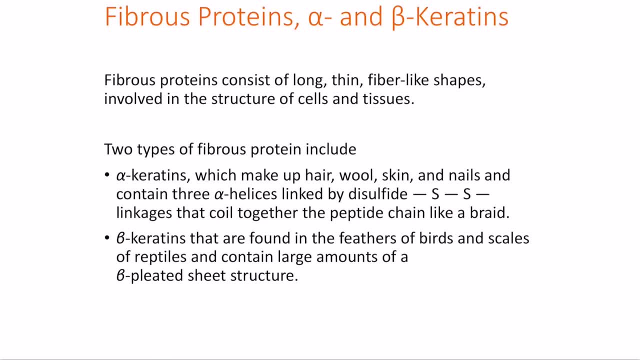 and it generally contains about 153 amino acids in a polypeptide structure, with about three-fourth of the chain in the alpha helix secondary structure. next you also have fibrous proteins such as alpha and beta carotenes. so fibrous proteins generally contain long, thin fiber-like shapes that are 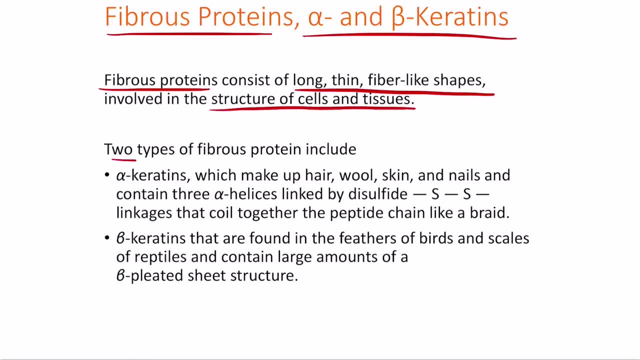 found in the structure of the cells and tissues. there are two types of fibrous proteins. one is alpha carotenes, the other is beta carotenes. alpha carotenes make up the hair, wool, skin and nails, and they generally contain three alpha helices that are linked by disulfide linkages that coil. 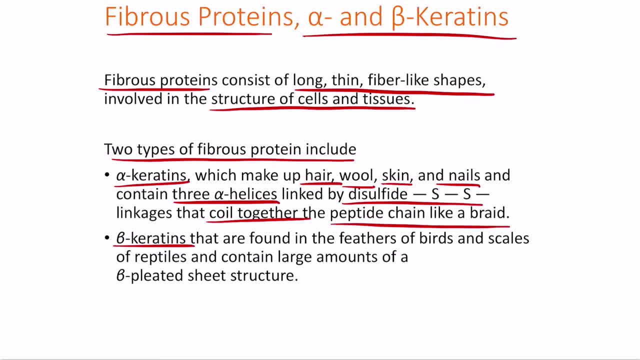 together the peptide chain like a braid right. so if you, if you have seen a braid braiding of your hair, that's an example of a fibrous alpha carotene structure. beta carotene is generally found in the feathers of birds and scales of reptiles. 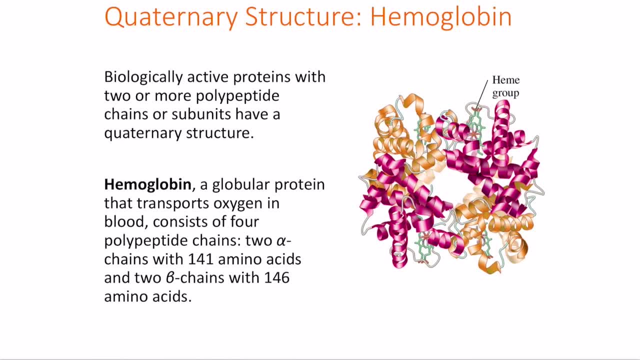 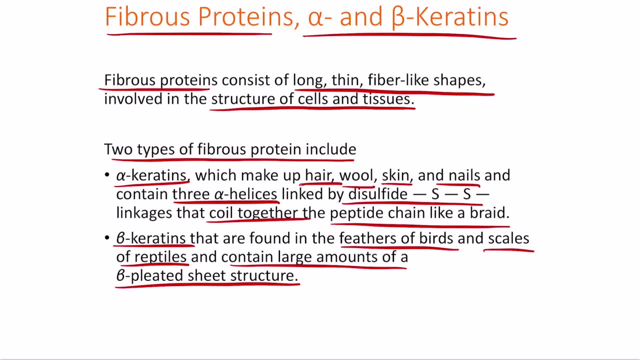 it generally contains large amounts of bleeder pleated seed structures. so the depending on the functioning. so, depending on the structure, the function varies as well. for example, alpha carotenes make up the structure of hair, wool, skin and nails. beta carotenes generally make up the beta sheets. 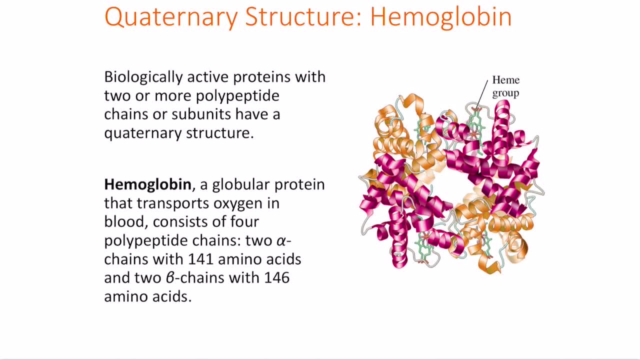 which are generally responsible for the feathers of birds and scales of reptiles. next, finally, we come to the quaternary structure, which is the example- let's take the example- of a hemoglobin- now biologically active proteins with two or more polypeptide chains or subunits, generally. 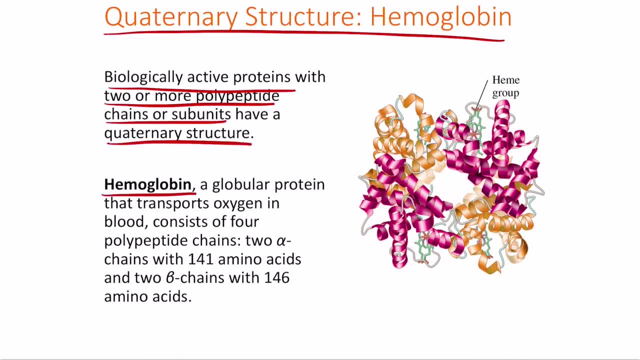 have a quaternary structure. for example, take- let's take- hemoglobin. hemoglobin is a globular protein that transports oxygen in blood and consists of four polypeptide chains. it has two alpha chains with 141 amino acids and two beta chains with 146 amino acids. 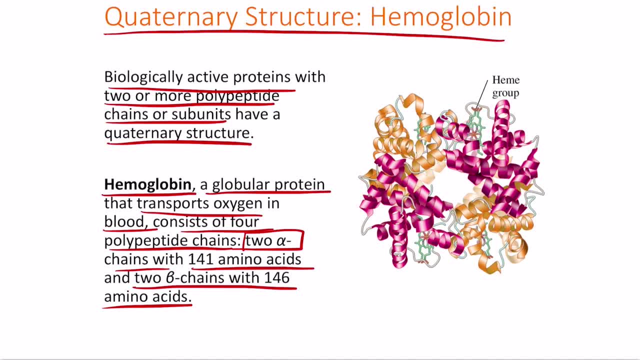 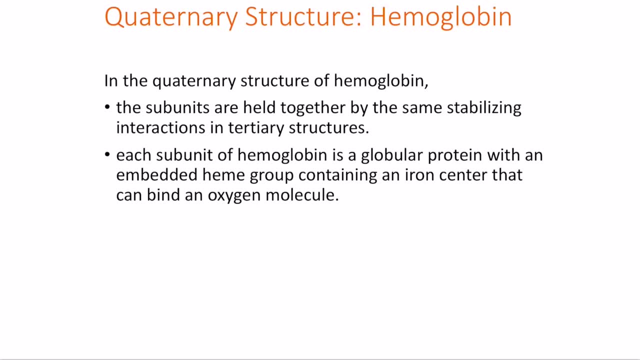 so this combined structure also contains a small ligand structure, so these are generally called ligands. ligands are small structures connected to the original protein, and these are ligands that are responsible for the quaternary structure of the protein. in the quaternary structures, these subunits are held together by the same stabilizing interactions. in the tertiary, 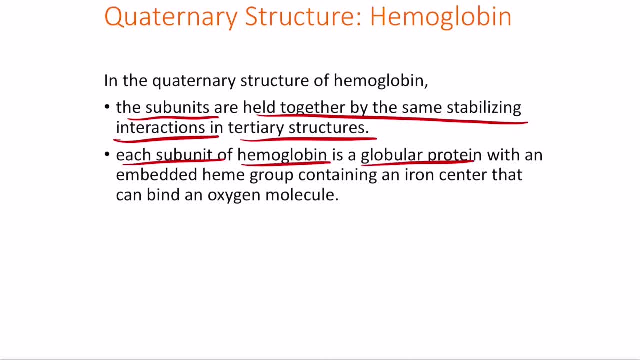 structures, but each subunit of the hemoglobin. here is a globular protein with an embedded heme heme group. notice that this is the external. this embedded heme group is also called as a ligand, and that ligand contains an iron center that can bind an oxygen molecule. this ligand, most commonly 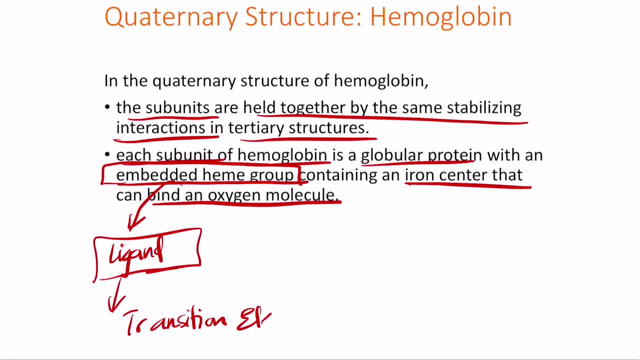 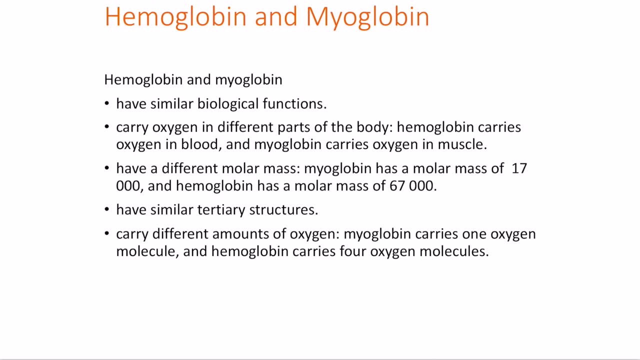 are transition compounds, so transition element complexes. so in common name we also call these the coordination compounds. so hemoglobin and myoglobin will have. they have the same biological function. they generally carry oxygen in different parts of the body. for example, hemoglobin carries oxygen in blood but myoglobin carries oxygen in the muscle they have. 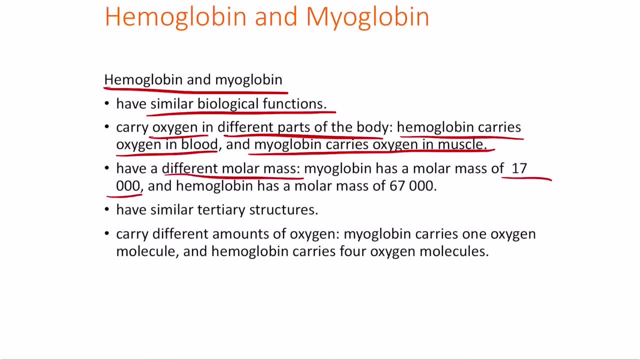 different molar masses. myoglobin has a molar mass of 17 000. hemoglobin has a molar mass of 67 000. they have really similar tertiary structures but they carry different amounts of oxygen, because myoglobin carries one oxygen molecule, whereas hemoglobin can carry four oxygen molecules. 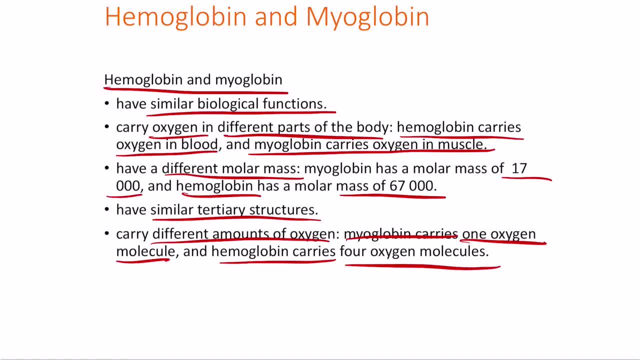 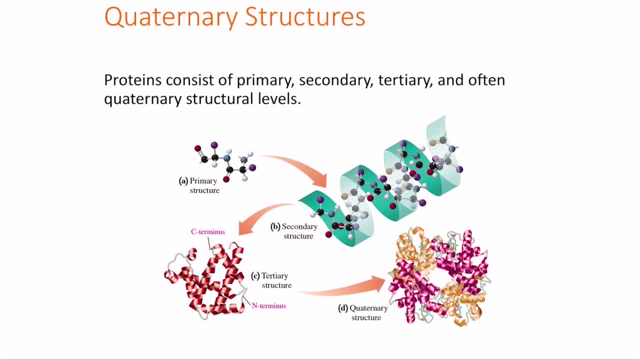 so the type of ligand and the number of ligands that are attached is representation of the quaternary structure of the protein. so proteins start from. they contain a protein called the. So they start from the primary, secondary, tertiary and often quaternary structural levels. 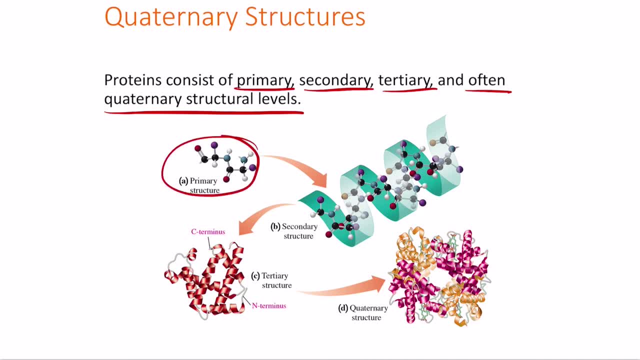 You start from a primary structure of linkages of amino acids and the secondary structure, which is the interactions between the residues of the amino acids and third, creating the interactions from the secondary structure, then create a three dimensional shape. The three dimensional shape, then, can embed external coordination complexes which create 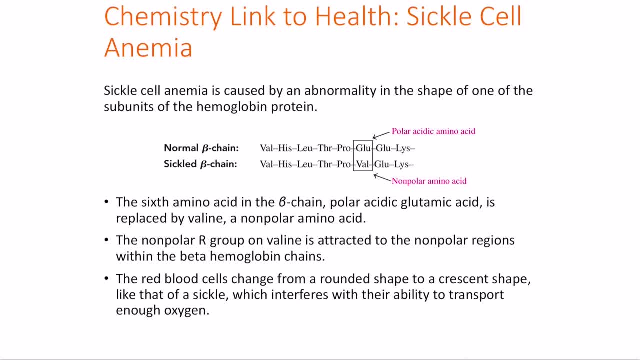 the quaternary structure of the protein. So let us talk about one of the main diseases that happens due to the abnormality of the hemoglobin protein, So, which is sickle cell anemia. So sickle cell anemia is caused by the abnormality in the shape of one of the subunits of the 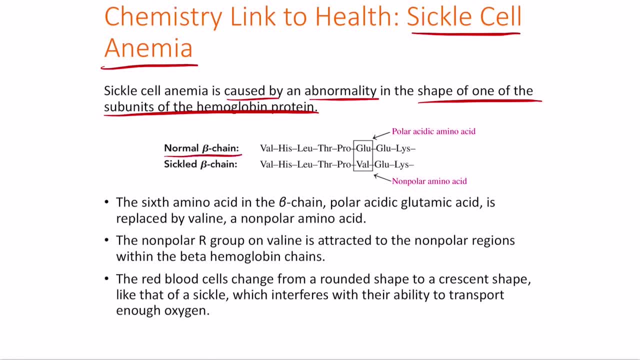 hemoglobin protein, For example, a normal beta chain in hemoglobin contains gluosein, but a sickled beta chain contains valine And this is a. This is a non-polar amino acid and but gluosein originally is a polar amino acid. 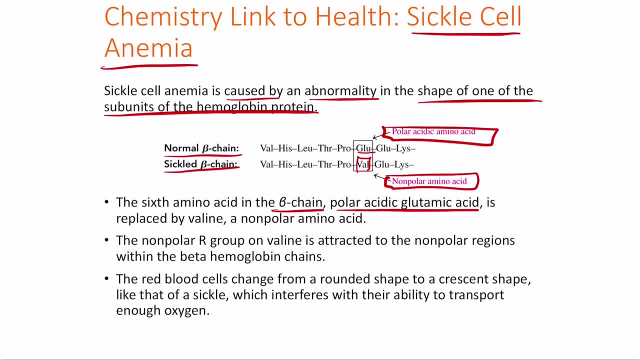 Now the sixth amino acid in the beta chain, which is the polar acidic glutamic acid, is replaced by a valine, a non-polar amino acid which creates the non-polar R group on. the valine is attracted to the non-polar regions within the beta hemoglobin chains. 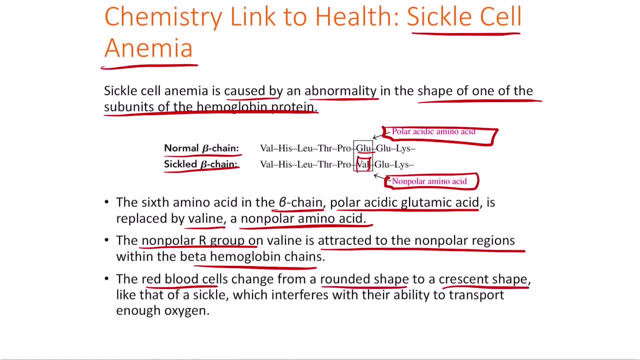 The red blood cells change from a rounded shape to a crescent shape. So that is the reason why we call it a sickle, Which interferes with the ability- The ability to transport enough oxygen. That is the reason why it ends up not having enough oxygen, which creates lesser energy. 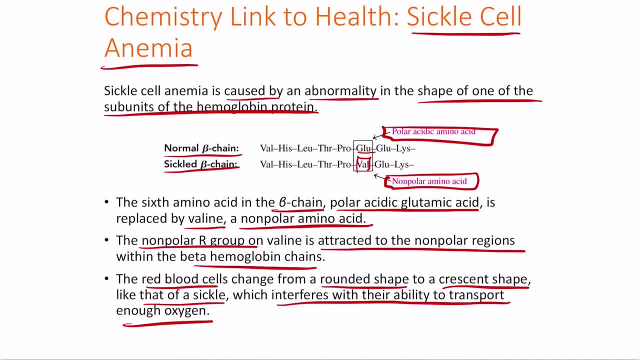 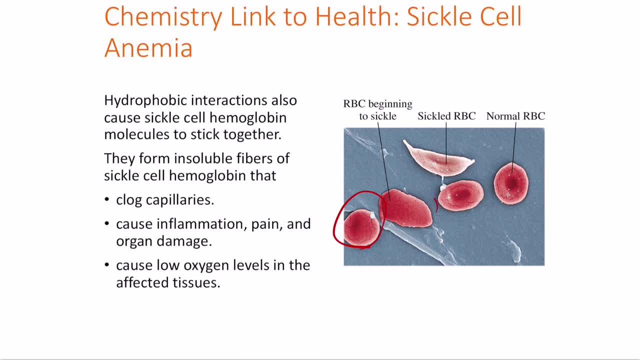 in the body which creates the structure which creates the anemic characteristics in the body. So this is a normal RBC and this is a structure that is beginning to sickle. and this is the completely sickled red blood cell. Notice the change in the normal red blood cell and a sickled red blood cell. 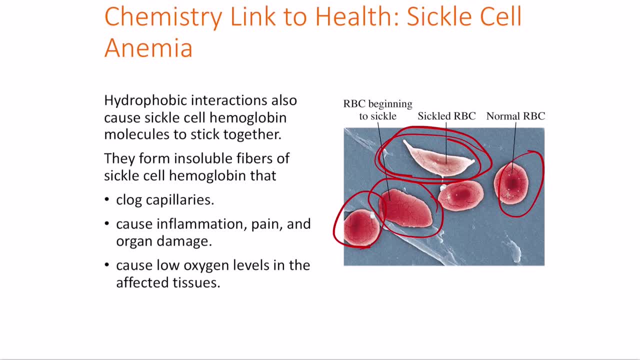 Notice the crescent structure. The crescent structure creates the problems here. So this is the red blood cell. This is the red blood cell. Now, these hydrophobic interactions can cause sickle cell and hemoglobin molecules to stick together. 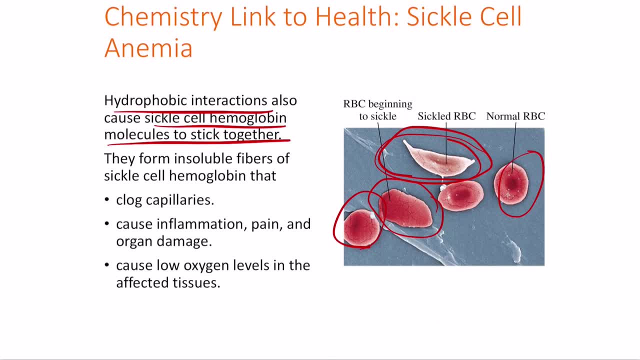 Now these hemoglobin hydrophobic interactions can cause the molecules to stick together and they form insoluble fibers of sickle cell hemoglobin that can clog capillaries. It can cause inflammation, pain and organ damage. It can also cause low oxygen levels in affected tissues. 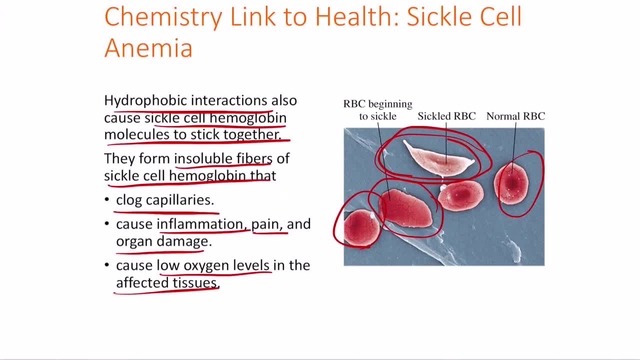 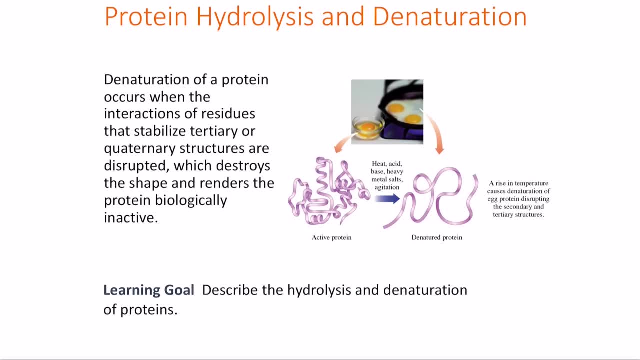 So this is the. This is the link between sickle cell anemia and the change in the structure of the hemoglobin, and how one single amino acid can result between a diseased red blood cell and an undiseased red blood cell. So next let us talk about the last topic: protein hydrolysis and denaturation. 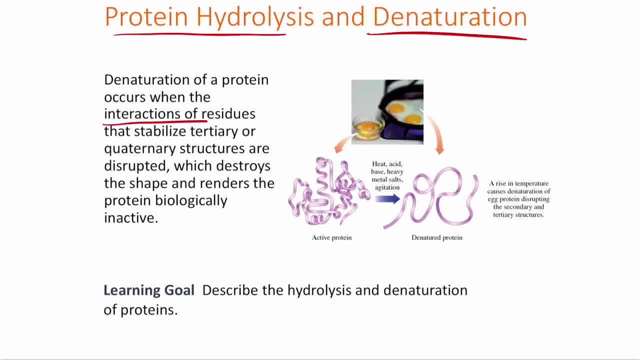 So what is the denaturation of a protein? It occurs when the interactions of the residues that stabilize the tertiary or quaternary structures are disrupted. We generally can destroy the shape and render the protein. So what is the denaturation of a protein? 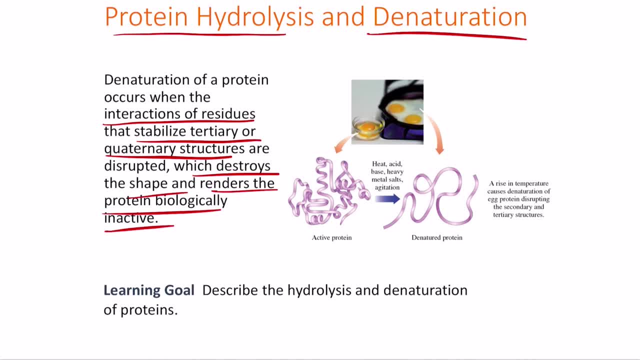 The denaturation is one of the characteristics of an amino acid that is first denatured and then the protein is later denatured and then the protein is released. We can call this denaturation the denaturation of a protein. Now, the denaturation of a protein can occur when the agent is released from the amino. 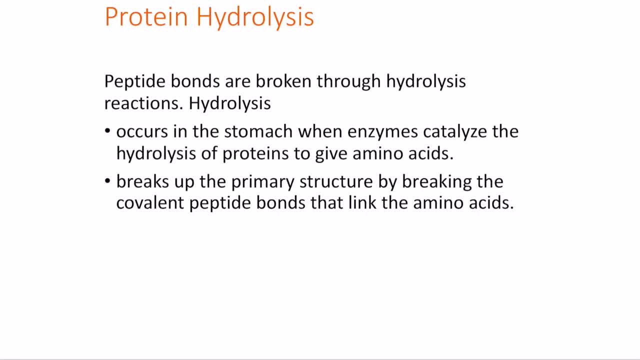 acid and is released from the protein. It is not an easy process but the reaction is often slow in its initial production. What is the denaturation of the protein? bonds here are generally broken through hydrolysis reactions. The reason? because we already talked about peptide bonds- are result of dehydrolysis, which means that when we remove dehydration, which means when we remove hydrogen water, it results in the formation of a peptide bond. So when you add water they end up becoming individual mono amino acids. So these generally occur in the stomach when enzymes catalyze the hydrolysis of proteins to give amino acids. 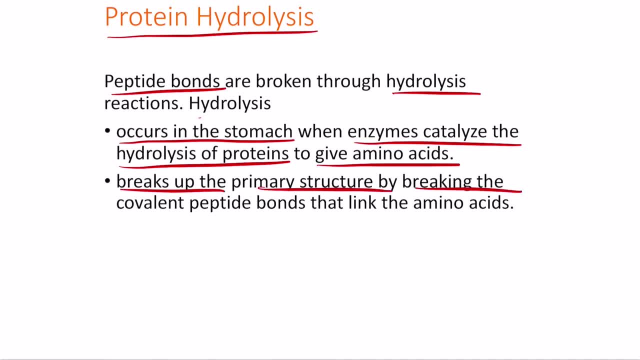 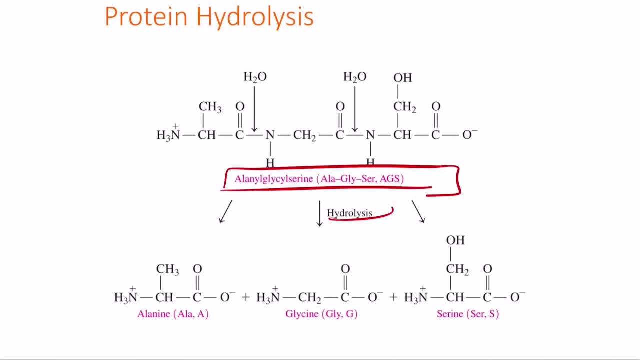 They break up the primary structure by breaking the covalent peptide bonds that lick the amino acids. So, for example, alanine glycyl, serine under hydrolysis can create alanine glycine and serine, So the combined structure. 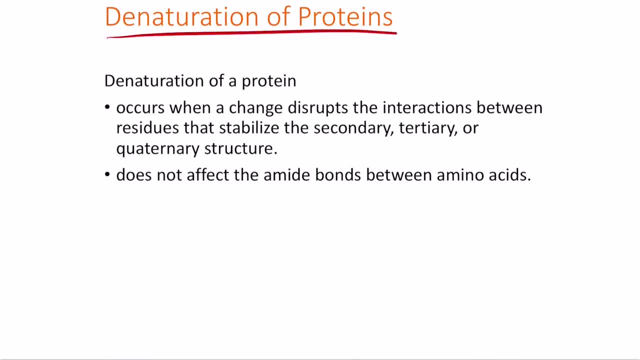 Next is denaturation of proteins. Denaturation occurs when a change disrupts the interaction between the residues that stabilize the secondary, tertiary or quaternary structures. Now, these originally do not affect the amino acid amide bonds between the amino acids. 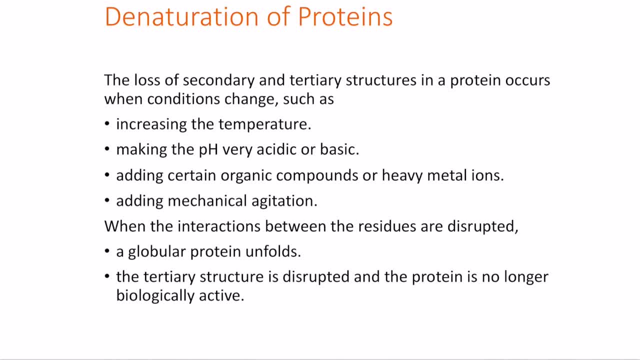 But rather affects the stabilizing bonds in the secondary structure of the protein. Now, the loss of this secondary and tertiary structure in the proteins occurs when conditions change. The conditions that change are: increase in the temperature, making the pH very acidic or basic, Adding certain organic compounds or heavy metal ions and adding mechanical agitation. 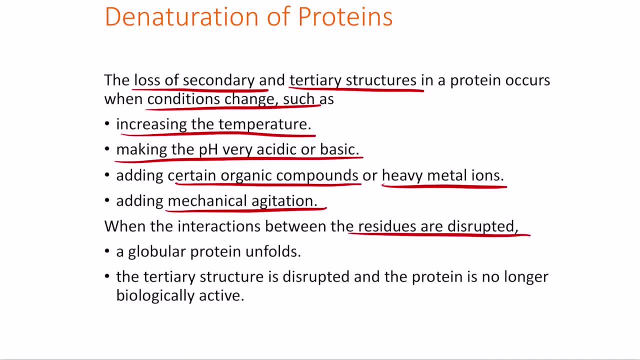 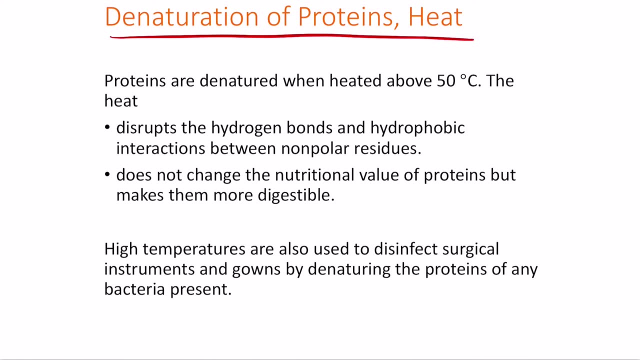 So when the interactions between the residues are disrupted, you can have unfolding of the globular proteins. The tertiary structure ends up disrupted and the protein is no longer biologically active. So the first out of these processes is heating. So proteins are generally denatured when you heat above 50 degree centigrade. 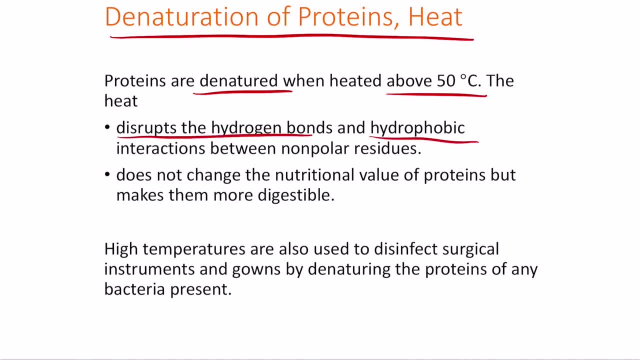 And the heat can disrupt the hydrogen bonds and the hydrophobic interactions between the whole non-polar residues. This does not change the nutritional value of the protein, but makes them more digestible. That's the reason why you actually heat up the protein. 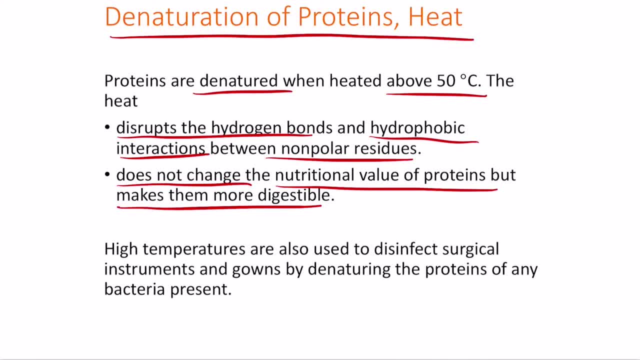 That's the reason why you actually heat up the protein Instead of taking the food directly into your own body. The reason why you cook food is because when you cook food, you are breaking up the individual proteins into their basic amino acids, primary or secondary structures. that increases the chance of digestion in your body. 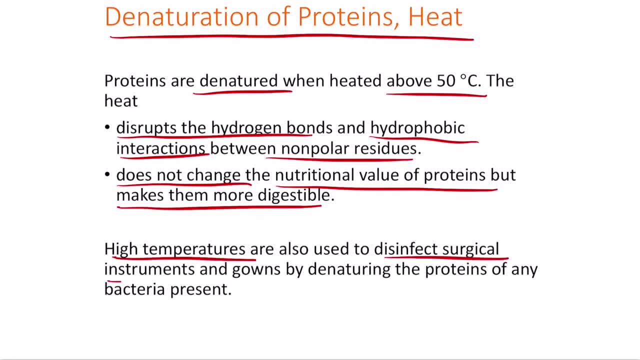 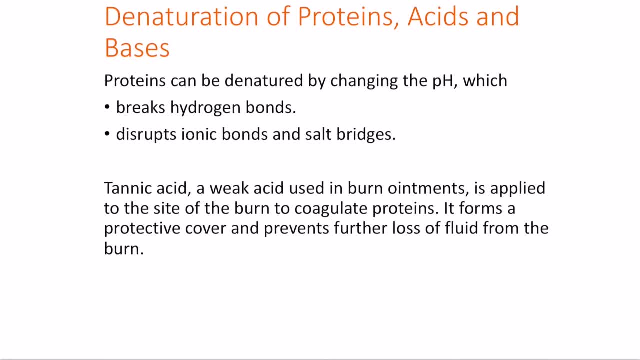 So high temperatures are also used to disinfect surgical instruments and gowns by denaturing the proteins of any bacteria that are present. This is how bacteria can die at high temperatures. Next is acids and bases. Proteins can also be denatured by changing the pH. 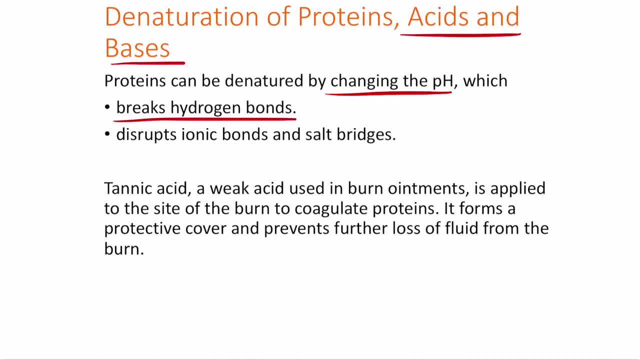 because changing the pH can break the hydrogen bonds and can also disrupt the ionic bonds and the salt bridges in the structure. For example, a tannic acid is a weak acid that is used in burn ointments When it's applied to the 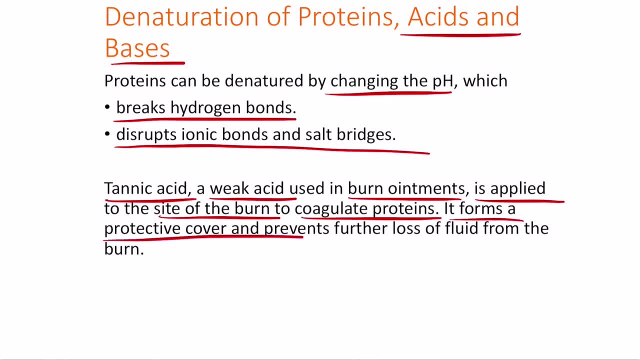 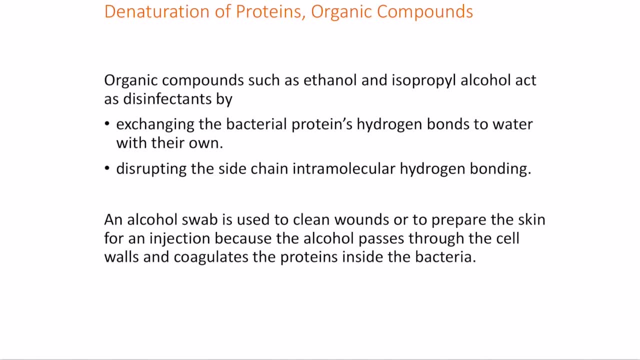 site of the burn to coagulate proteins. it forms a protein cover, protective cover- and prevents further loss of fluid burns. Next is organic compounds. so organic compounds such as ethanol and isopropyl alcohol can act as disinfectants by exchanging the bacterial proteins hydrogen bonds to 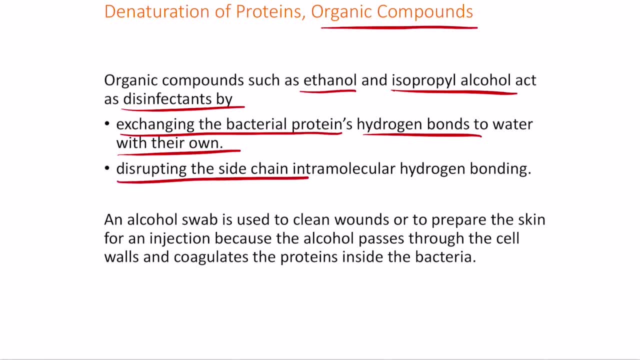 water with their own. and second is disrupting the side chain intramolecular hydrogen bonding. so when you use an alcohol swab to clean a wound or to prepare the skin for an injection, we generally do that because the alcohol passes through the cell walls and coagulates the proteins. 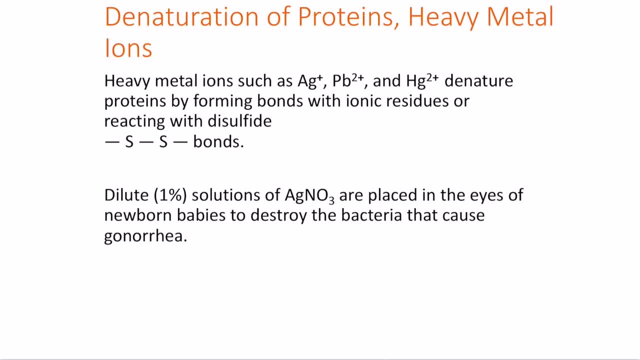 that are inside the bacteria. Next is heavy metal ions. Heavy metal ions, such as silver, lead and mercury, can denature proteins by forming bonds with the ionic residues or reacting with the disulfide bonds, For example, a dilute solution of silver nitrate. when you placed in the eye of a 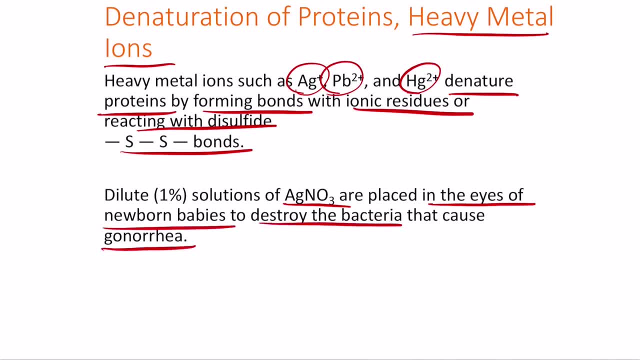 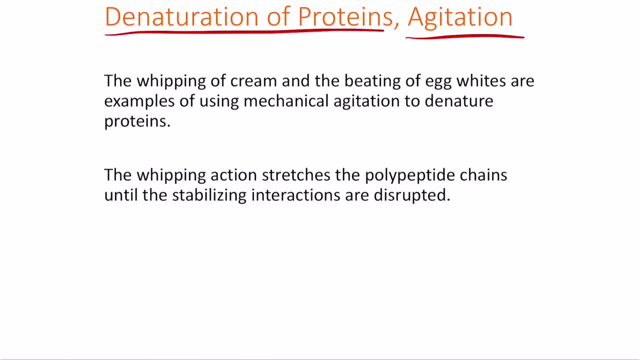 newborn baby to destroy the bacteria that causes gonorrhea. So denature of proteins can also be created by agitation. For example, the whipping of cream and the beating of egg whites are natural examples of using mechanical agitation to denature the proteins. So it unfolds the primary structure. 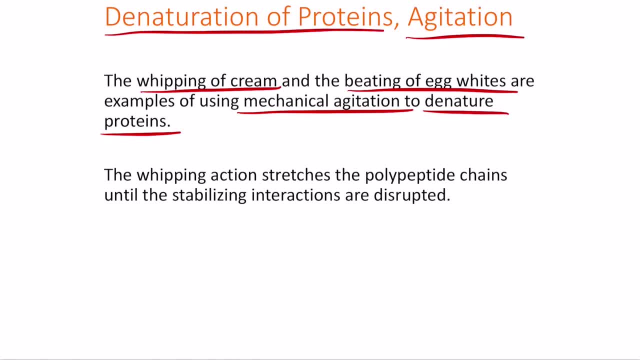 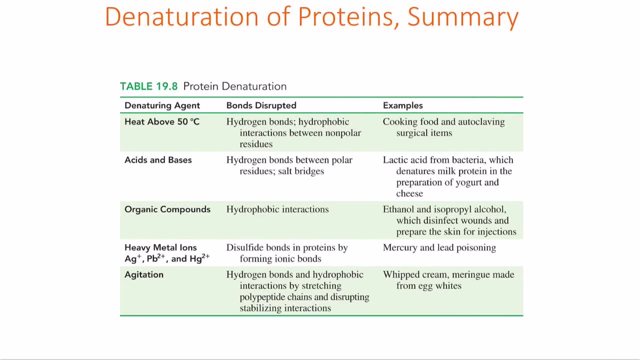 of the protein and resulting in the expansion of the original structure. Now, for example, the whipping action basically stretches the polypeptide chains until the stabilization interaction happens. So these are the four things that can be done. Heating above 50 degrees ends up breaking the 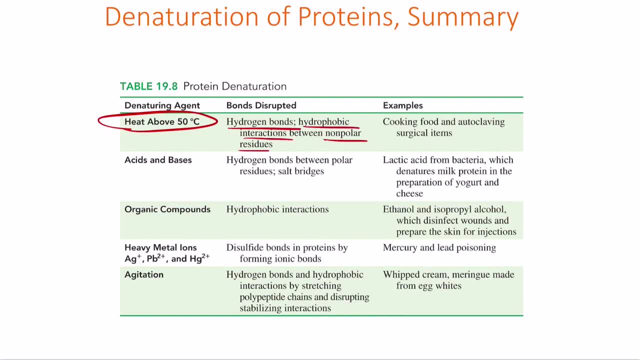 hydrogen bonds, hydrophobic interactions between the non-polar residues. Examples of this are cooking food, autoclaving and surgical items. You have acids and bases. This generally disrupts the hydrogen bonds between the polar residues and they also destroy the salt bridges. Examples of these: 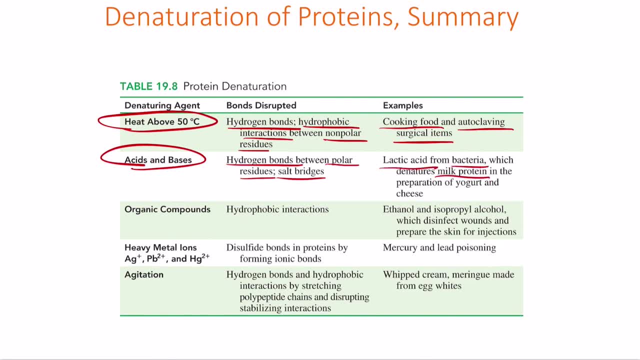 is lactic acid from bacteria, which denatures the milk protein. in the preparation of yogurt and cheese, You have organic compounds that can disrupt the hydrogen bonds. So these are the four things that can be done. So these are the four components, such as that they generally disrupt the hydrophobic interactions. 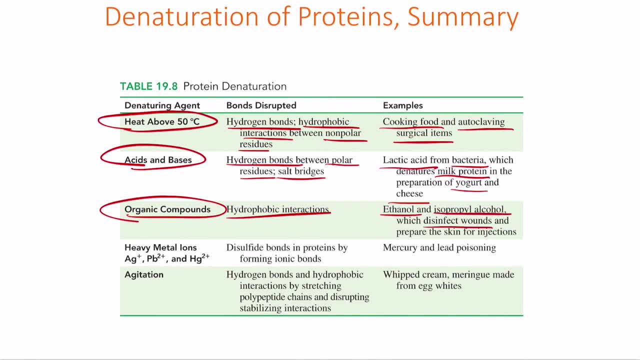 For example ethanol and isopropyl alcohol, which are used to disinfect wounds and prepare skin for injections, help in the removal or breaking of the cell walls of bacteria. Hemimetallions are generally disrupt the disulfide bonds in proteins by forming ionic bonds.